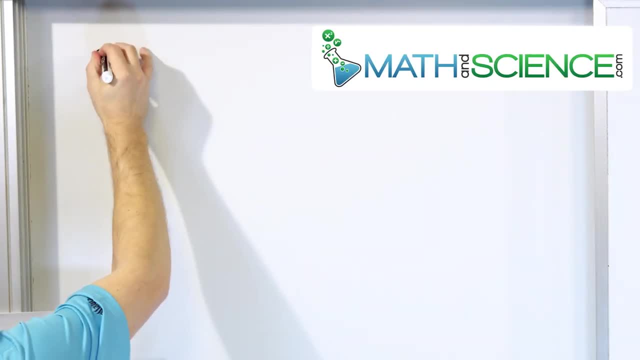 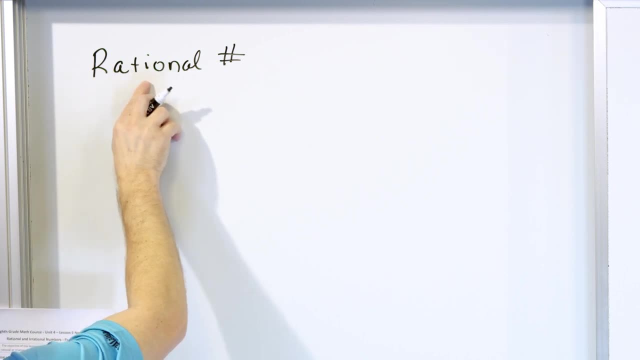 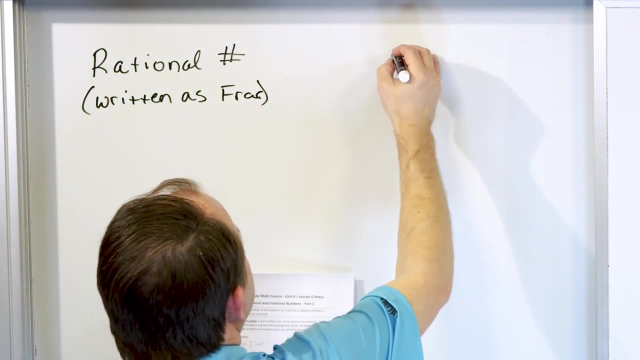 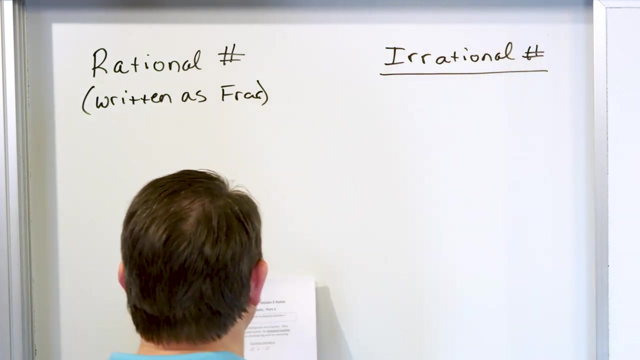 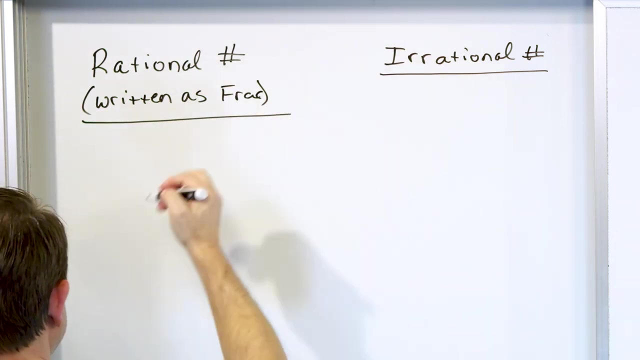 So remember rational number. It's spelled like this: rational number- Notice that the word ratio is inside of the word right, And so what rational number is is can be written as fraction, right Fraction, like this: And what about irrational? And these are numbers that cannot be written as a fraction. So let's give a couple of examples of each of these guys and then we'll solve a couple quick problems. Very simple concept, nothing hard here. 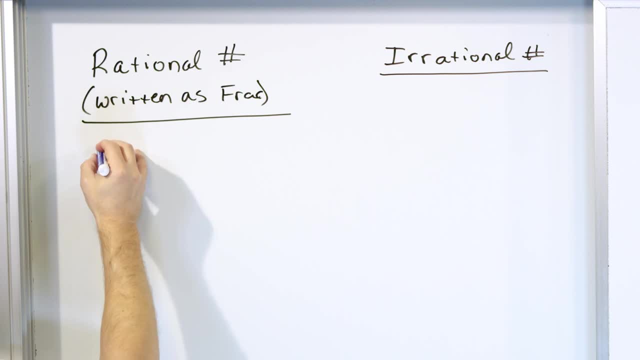 All right, rational number. What about all the whole numbers that you know, the number four, the number three and so on? Is the number four a rational number? All you have to do is say: can it be written as a fraction? 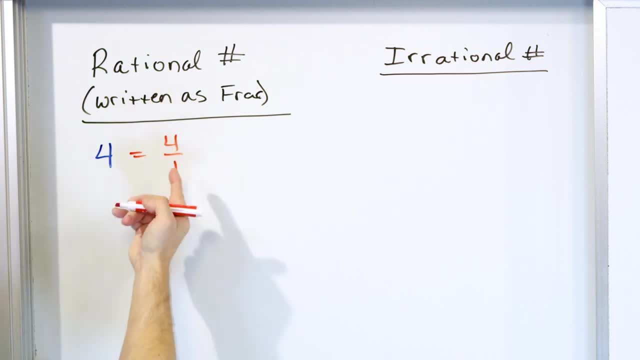 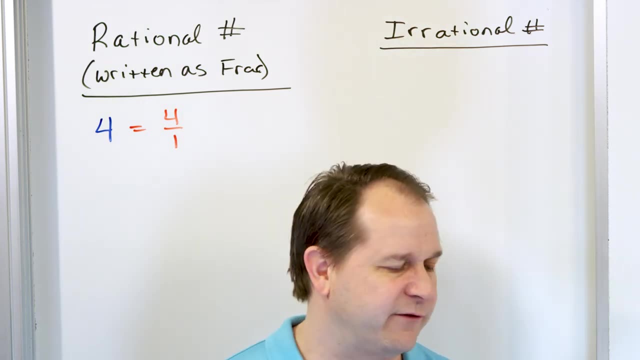 Well, the whole number four can be written as four over one. That's a fraction, And any whole number that you know can be written as a fraction. Ten can be written as ten over one. Twenty-five can be written as twenty-five over one. 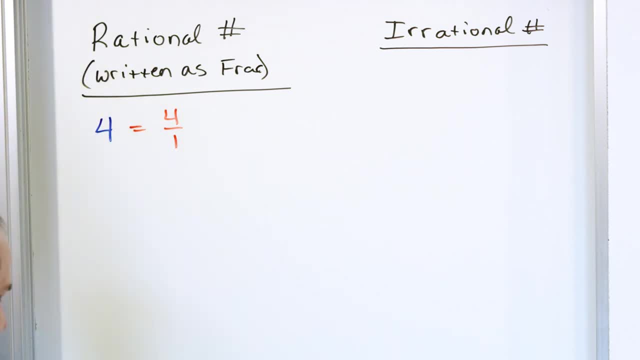 So all the whole numbers that you know are all rational numbers. All right, what about some of these other numbers, like negative numbers? What about negative two? Well, is this rational? All you have to do is say: can it be written as a fraction? You can write it as negative, two over one. So all the negative numbers, all the positive numbers, are all rational numbers. 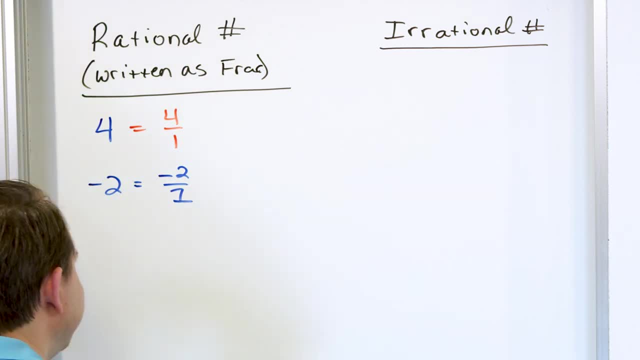 All right. What about the number zero? Is zero a rational or an irrational number? Well, zero can be written as lots of different things. You can write it as zero over two, Remember zero divided by two. zero divided by anything is zero. So I could write this as zero over two or zero over 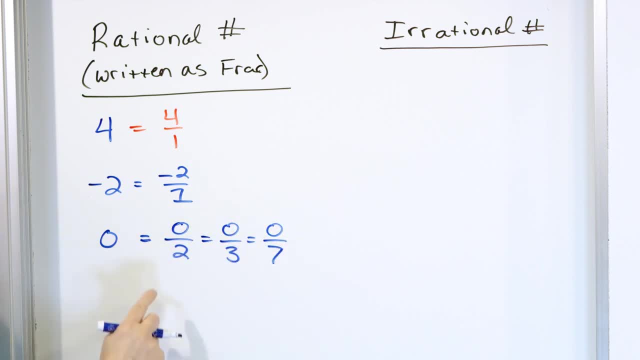 three, or zero over seven or whatever zero over anything, But anyway, these are all fractions. So zero is a rational number. All right, What about the number 1.25?? Okay, It looks like this is not a. maybe this is not a rational number, but it actually is, Because the number 1.25 can be. 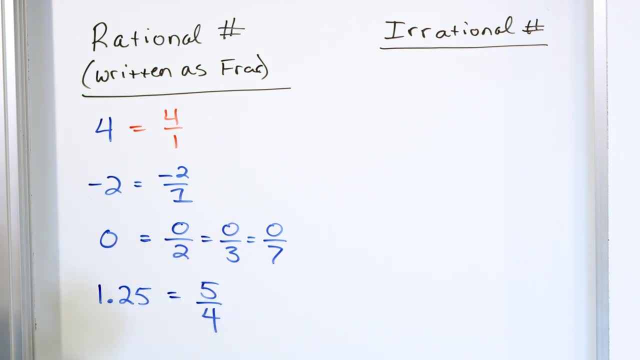 written as five-fourths, Because think about this number here, five-fourths, If you put it as a mixed number, divided in it goes one and one-fourth time. So one goes in one time with a remainder of one. five minus four is one. 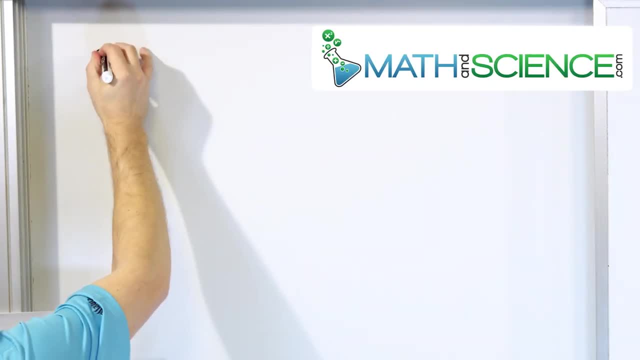 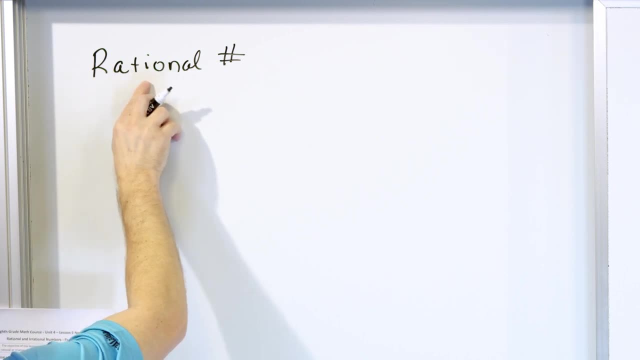 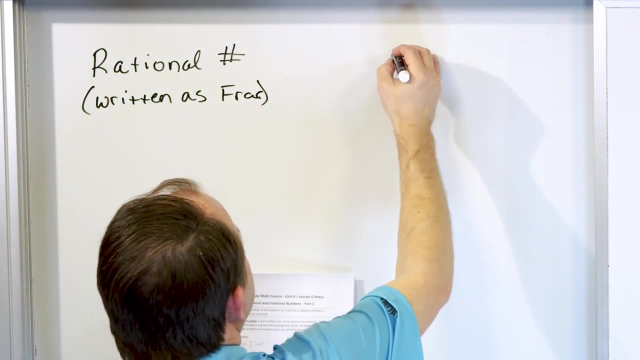 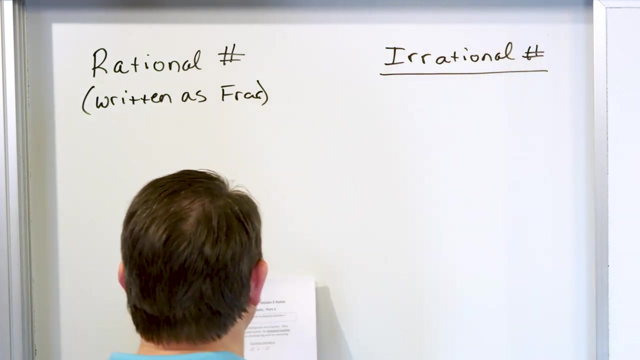 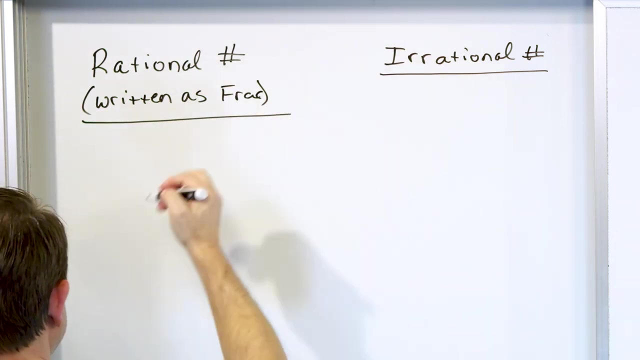 So remember rational number. It's spelled like this: rational number- Notice that the word ratio is inside of the word right, And so what rational number is is can be written as fraction, right Fraction, like this: And what about irrational? And these are numbers that cannot be written as a fraction. So let's give a couple of examples of each of these guys and then we'll solve a couple quick problems. Very simple concept, nothing hard here. 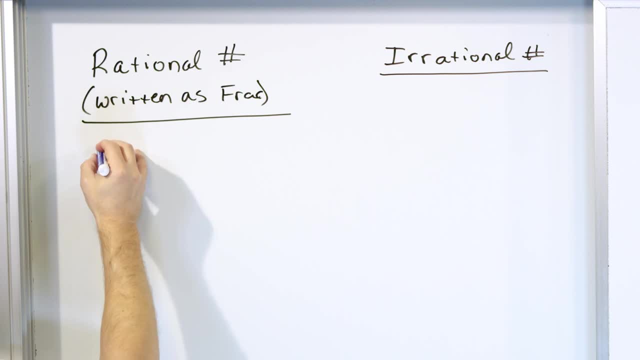 All right, rational number. What about all the whole numbers that you know, the number four, the number three and so on? Is the number four a rational number? All you have to do is say: can it be written as a fraction? 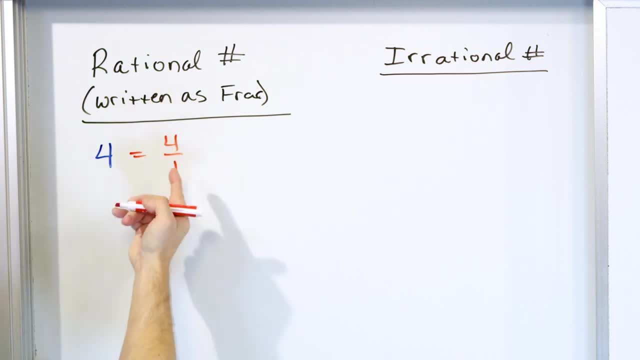 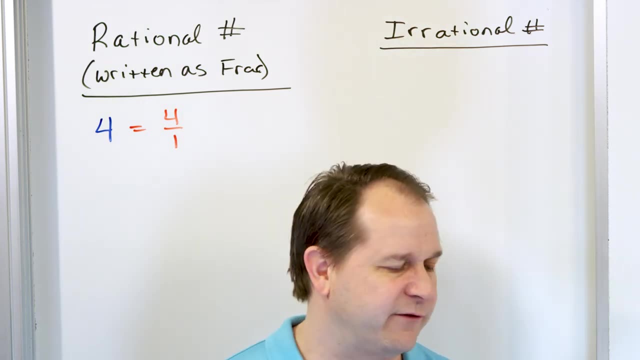 Well, the whole number four can be written as four over one. That's a fraction, And any whole number that you know can be written as a fraction. Ten can be written as ten over one. Twenty-five can be written as twenty-five over one. 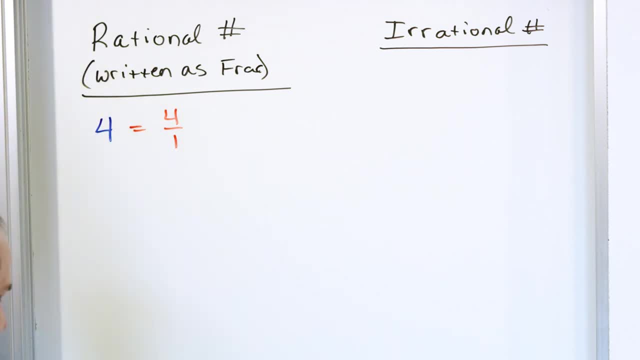 So all the whole numbers that you know are all rational numbers. All right, what about some of these other numbers, like negative numbers? What about negative two? Well, is this rational? All you have to do is say: can it be written as a fraction? You can write it as negative, two over one. So all the negative numbers, all the positive numbers, are all rational numbers. 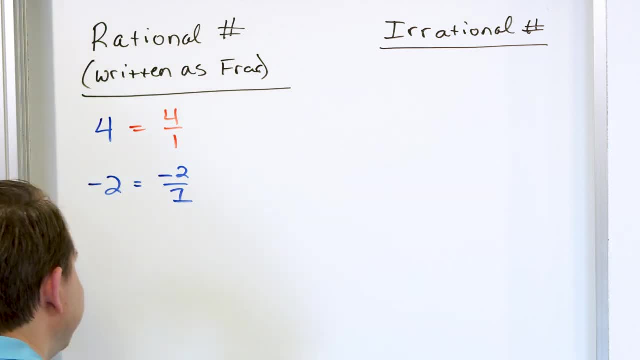 All right, what about the number zero? Is zero a rational or an irrational number? Well, zero can be written as lots of different things. You can write it as zero over two, Remember zero divided by two. zero divided by anything is zero. So I could write this as zero over two, or zero over three, or zero over seven, or whatever, Zero over anything. But anyway, these are all fractions. So zero is a rational number. 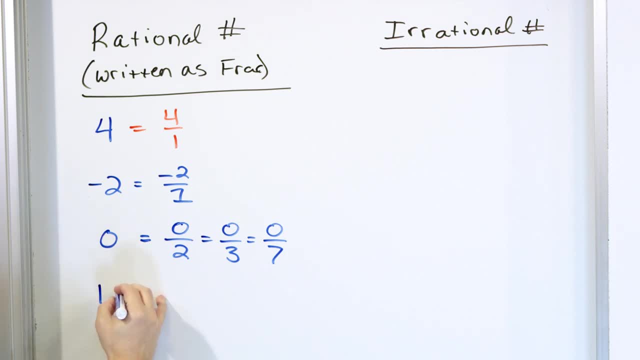 All right. what about the number 1.2?? Okay, it looks like this is not a. maybe, this is not a rational number, but it actually is, Because the number 1.25 can be written as five-fourths, Because- think about this number here- five-fourths, If you put it as a mixed number, divide it in, it goes one and one-fourth time. So one goes in one time, with a remainder of one. five minus four is one over four, So one and a fourth is like this: 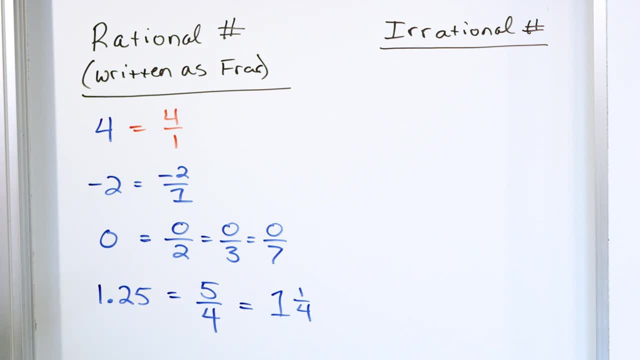 Over four. So one and a fourth is like this: It turns out that any of the decimals that you know, the decimals that you get in a calculator or just in calculations, they're almost always going to be rational. Either they're going to stop and the number, the decimals, are going to stop, like this: 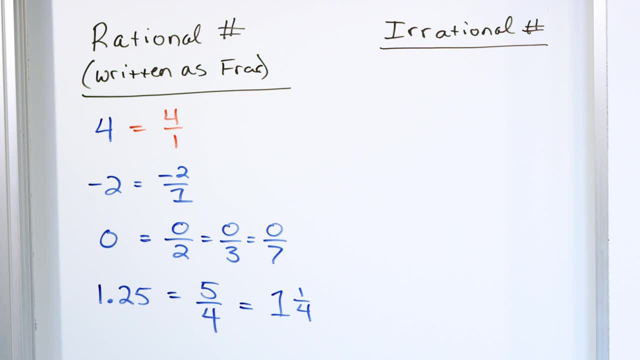 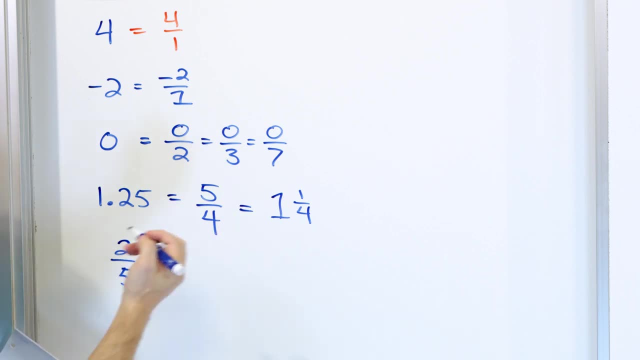 1.25, it stops. These can always be written as a fraction, And so they're all rational, All right. Of course, any of the actual fractions that you know, like two-fifths, can be written as a fraction, because it is a fraction. 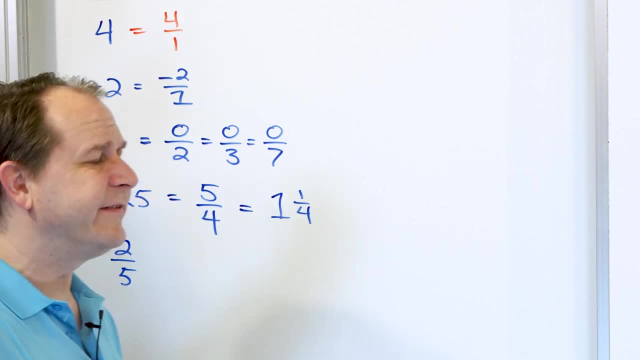 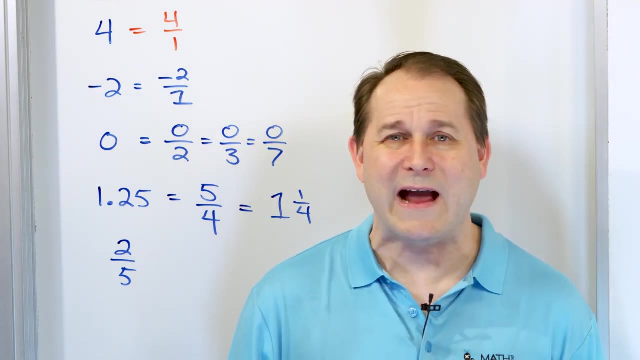 So all the fractions you know are rational. So you can see so far where you're kind of thinking what's left, Because I've told you, all the positive whole numbers are all rational, All the negative whole numbers are all rational, Zero's rational right, All the fractions that you know. one-fifth, 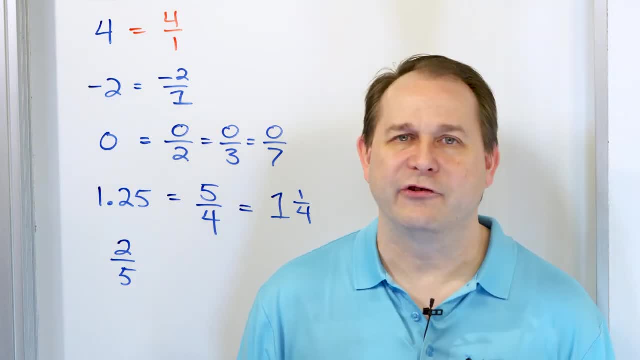 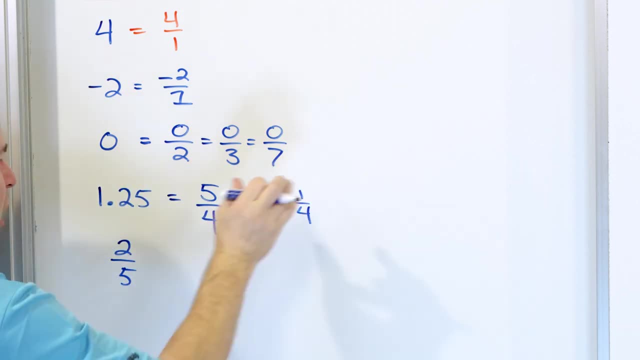 two-sevenths, three-eighths, they're all rational. All the negative fractions, they're all rational too. And all the decimals that stop and don't go on and on forever. they don't go on and on, they just truncate like this. 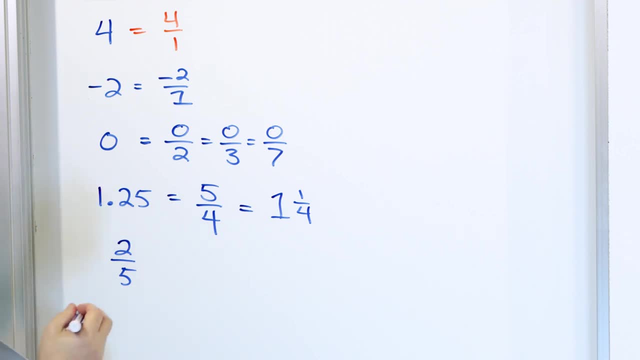 So it's good to be able to make those decisions in your own wrong thought process too. Okay, now let's talk about the rational part. So this is not the rational part, right? I really want my decimals to be written as a fraction too, So they're all rational as well. 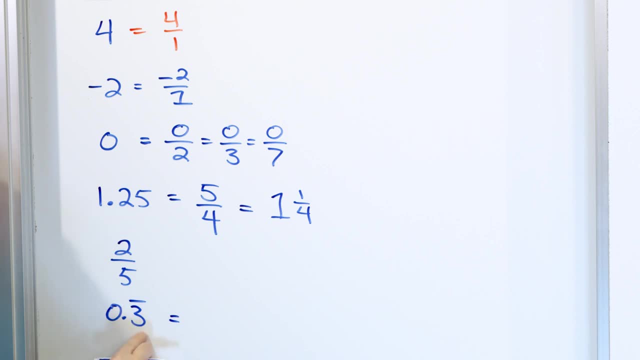 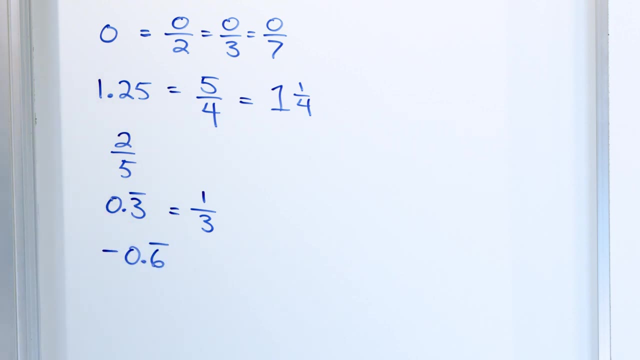 And what about? you know things like 0.3 with a repeating bar. This is 0.333333333333.. Well, you might think that's not rational, but actually this decimal can be written as 1,3.. Right. What about negative 0.6? with a repeating bar over this? So this is like negative 0.666666666666666666666666666666666666666666666666666666666666666666666666666666666666666666666666666666666666666, like this: 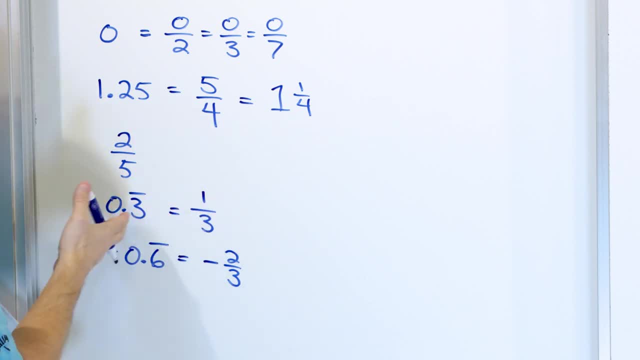 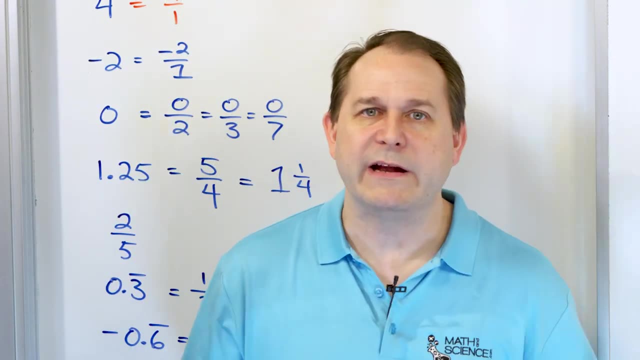 You can write this as negative two-thirds, So some of these fractions also can. these decimals that go on and on forever can be written as fractions. And here's the rule of thumb: If the decimal stops it can be written as a fraction. If the decimal goes on and on forever but it has a repeating pattern to it, 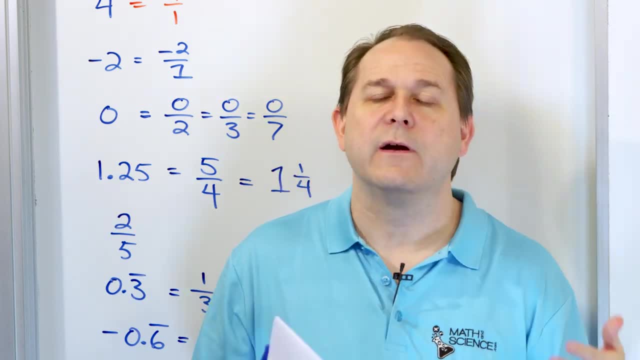 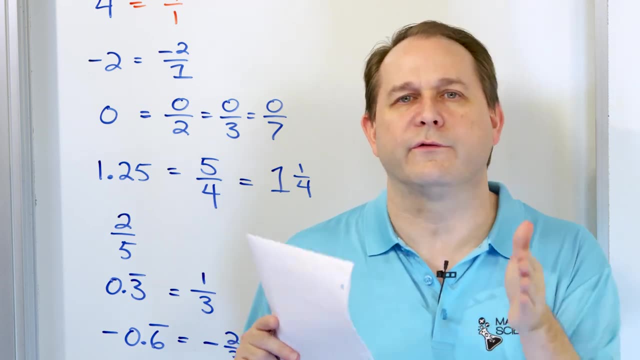 like 0.333333, on and on forever, then it's rational. It can be written as a fraction If there's any kind of pattern right in the decimals, even if it's like 0.123123123123123123123,. 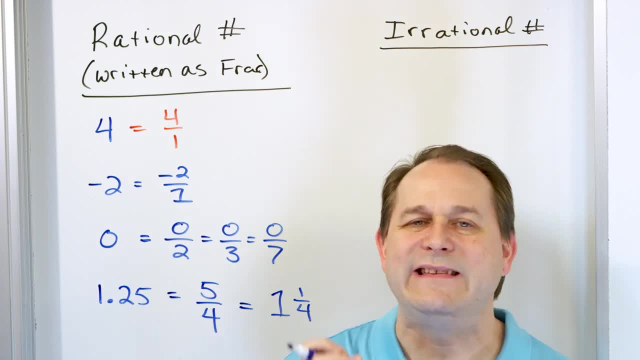 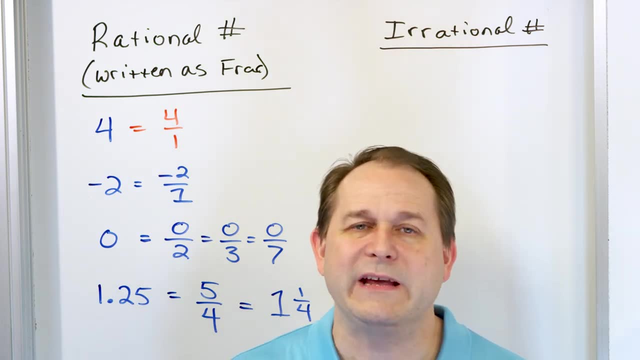 It turns out that any of the decimals that you know, the decimals that you get in a calculator or just in calculations, they're almost always going to be rational: either they're going to stop and the number, the decimals are going to stop, like this: 1.25, it stops. These can always be written as a fraction, and so they're all rational. 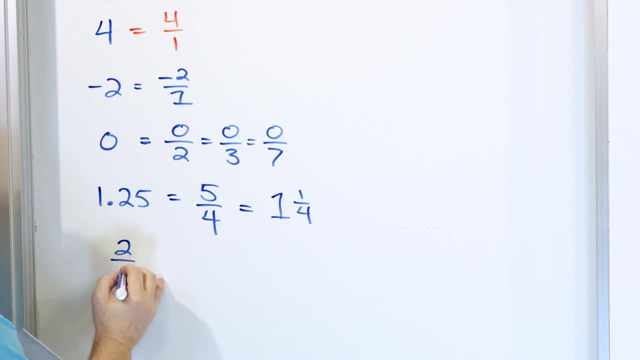 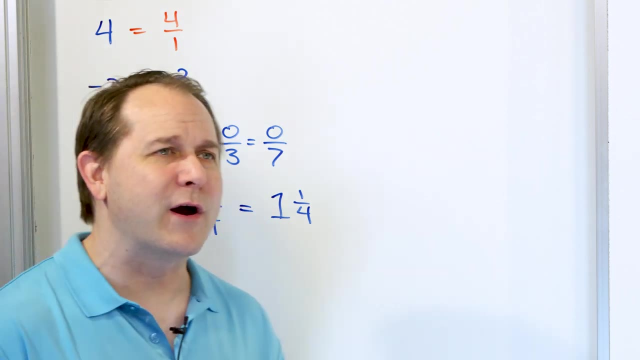 All right, of course, any of the actual fractions that you know, like two-fifths, can be written as a fraction because it is a fraction. So all the fractions you know are are rational. So you can see, so far we're kind of thinking about this as a rational number. 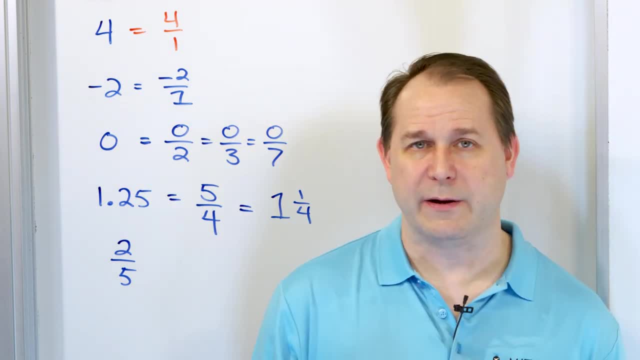 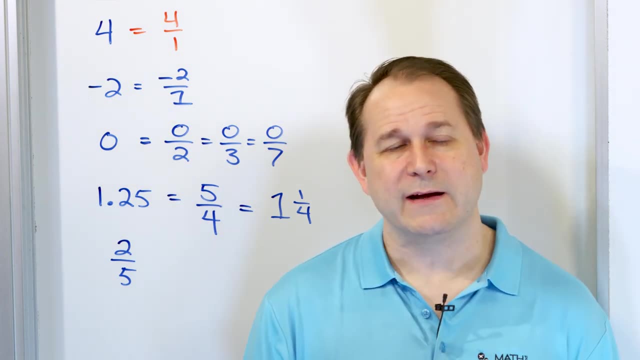 you're kind of thinking what's left? Because I've told you, all the positive whole numbers are all rational. All the negative whole numbers are all rational, Zero's rational right, All the fractions that you know, one-fifth, two-sevenths, three-eighths, they're all rational, All the. 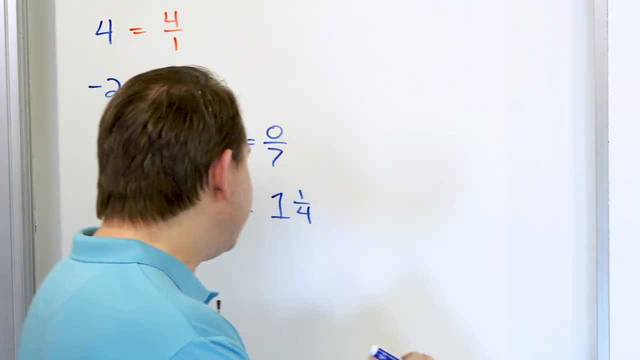 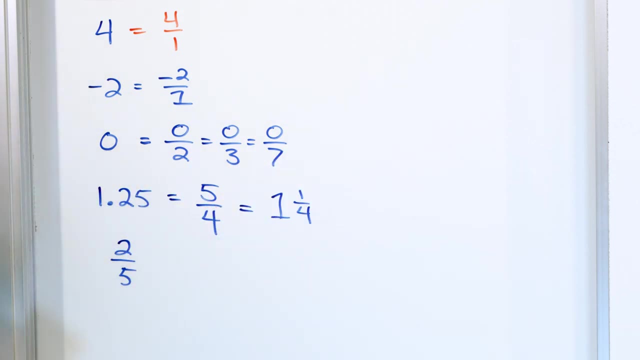 negative fractions. they're all rational too. And all the decimals that stop and don't go on and on forever. they don't go on and on, they just truncate. like this, they can always be written as a fraction too, So they're all rational as well. And what about? you know things like 0.3. 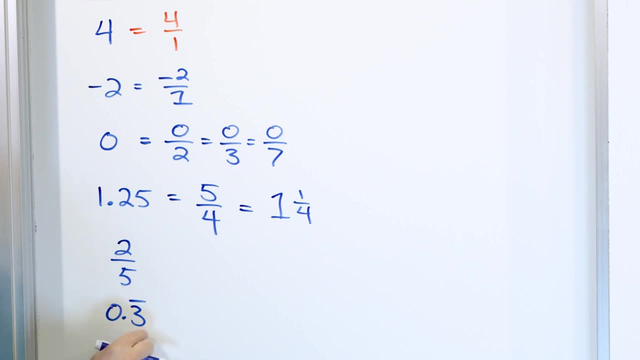 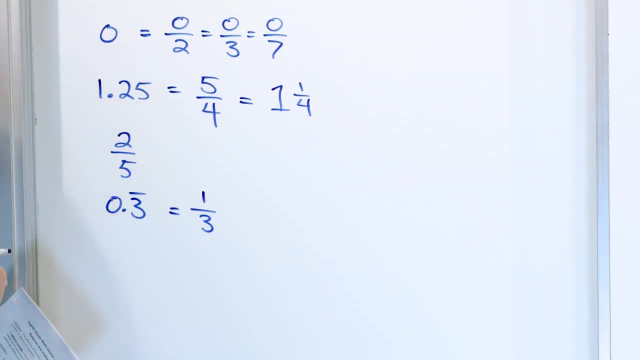 with a repeating bar. This is 0.3333333333.. Well, you might think that's not rational, but actually this decimal can be written as one-third right? What about negative 0.6 with a repeating bar over this? So this is like negative 0.6666666. like this, You can write this as negative two-thirds. 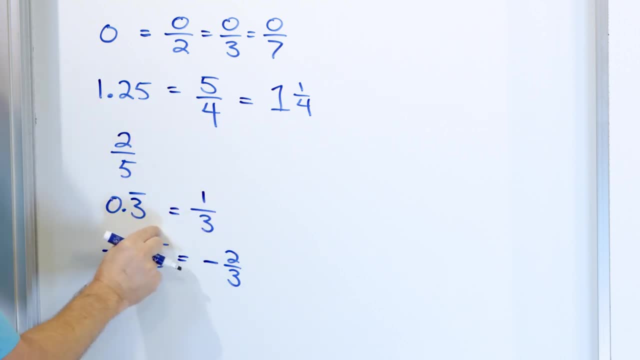 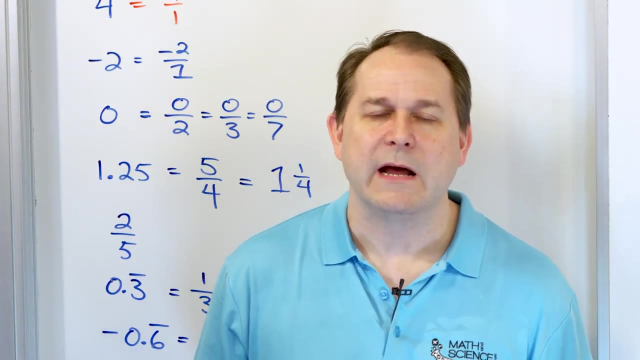 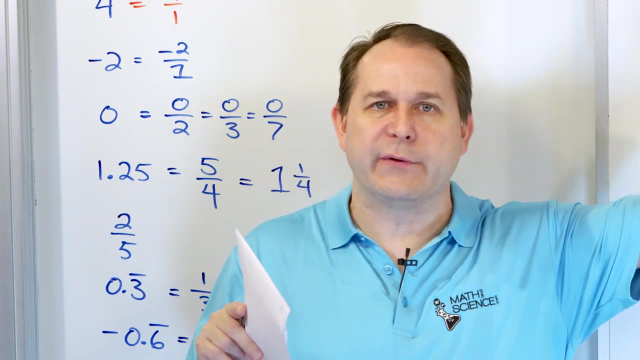 So some of these fractions also can, these decimals that go on and on forever can be written as fractions. And here's the rule of thumb: If the decimal stops it can be written as a fraction. If the decimal goes on and on forever but it has a repeating pattern to it, like 0.33333333- 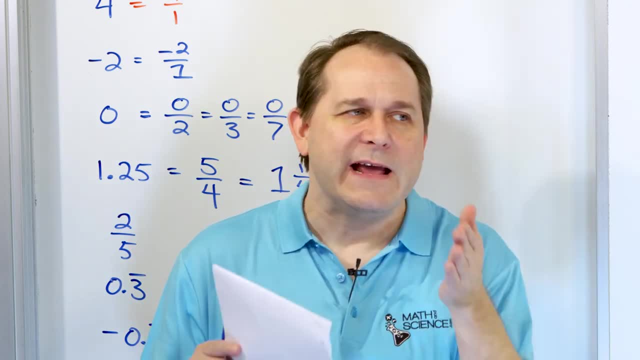 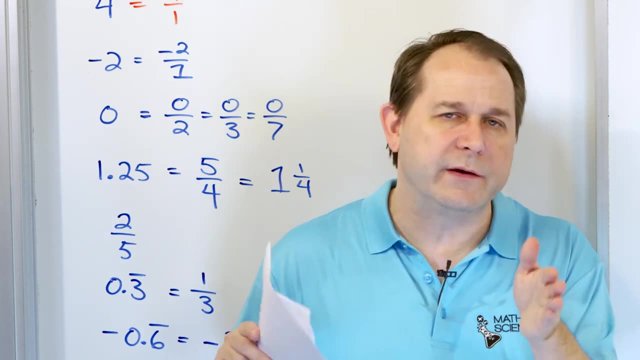 on and on forever, then it's rational. It can be written as a fraction. If there's any kind of pattern right in the decimals, even if it's like 0.123123123123123123123,, there's a fraction. So if the decimal stops, it can be written as a fraction. 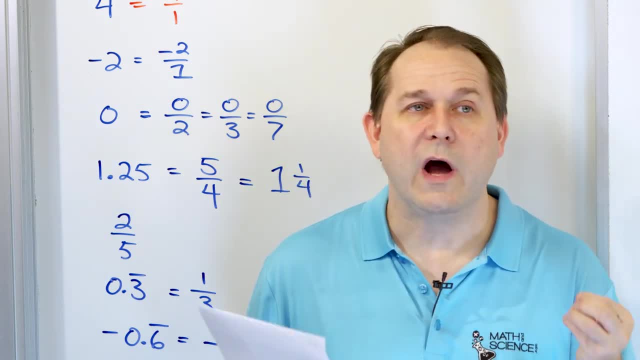 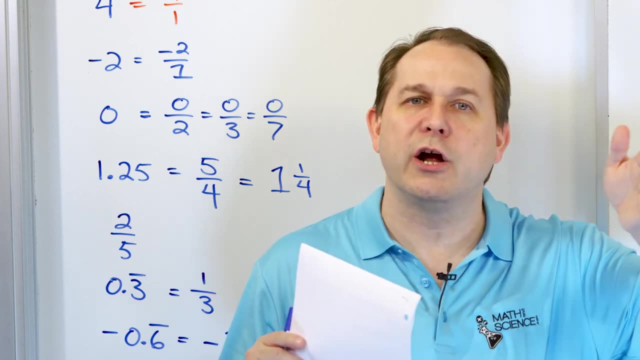 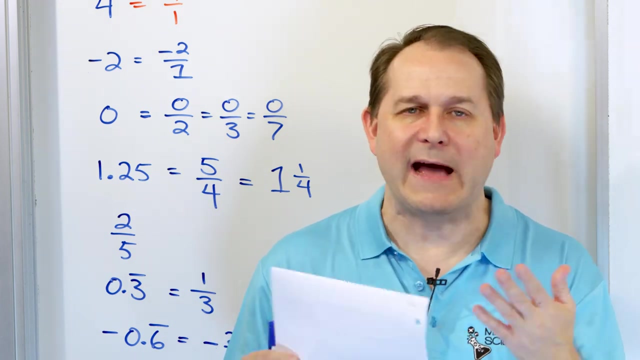 If there's a pattern, it can be written as a fraction, right? So what are the numbers that are irrational Then? the only way that you can have those, basically, is if the decimals go on and on forever and there is no pattern to them. So again, 0.123123123,. that is rational because 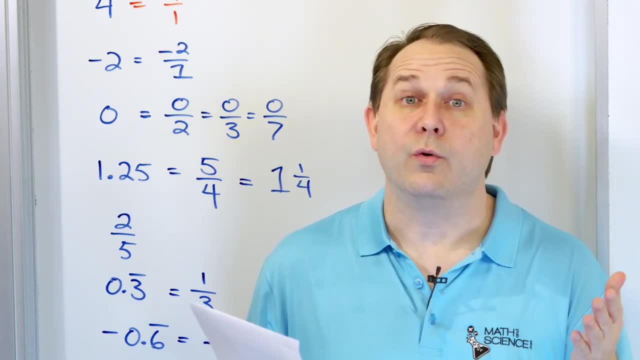 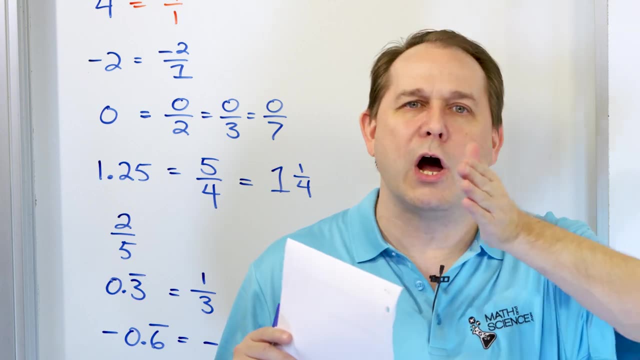 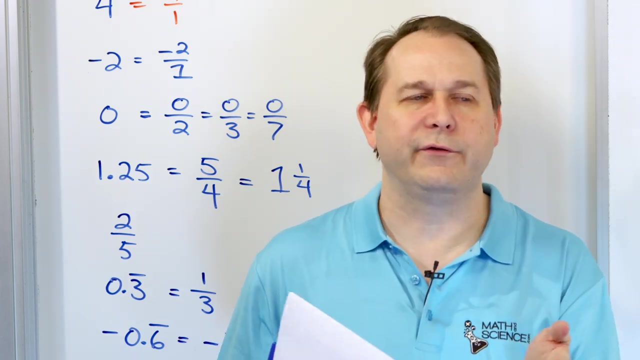 there's a pattern. it can be written as a fraction, right? So what are the numbers that are irrational Then? the only way that you can have those basically is if the decimals go on and on forever and there is no pattern to them. So again, 0.123123123,. that is rational because 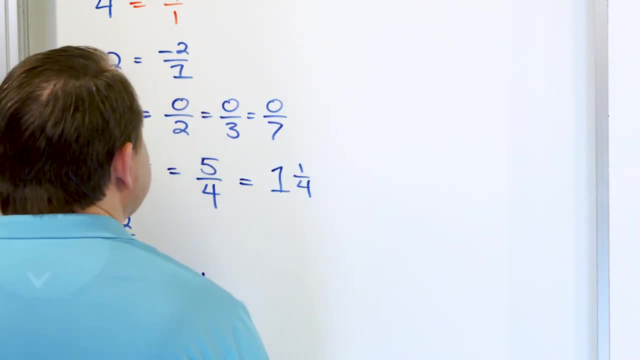 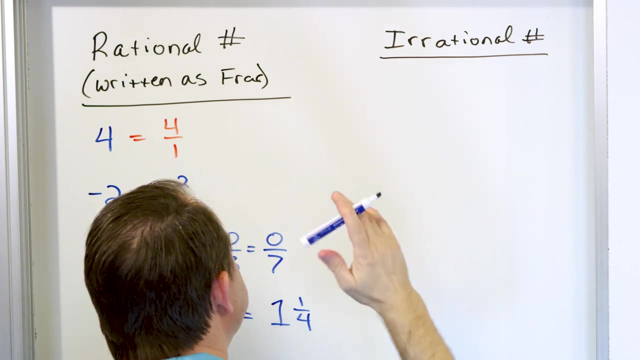 there's a pattern. So let's give some examples of the, some numbers that are irrational. Well, the most famous one that you're all aware of, the, the, the granddaddy of all of them, is the number pi. Some people may have told you incorrectly. 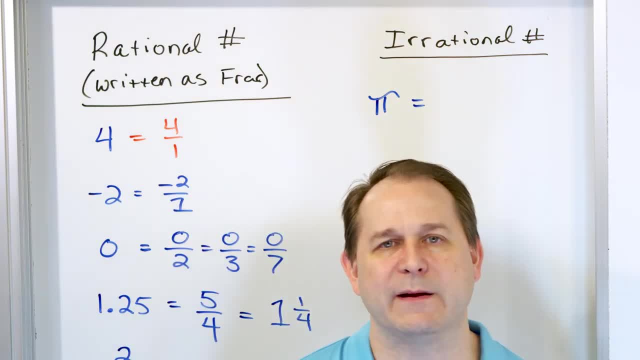 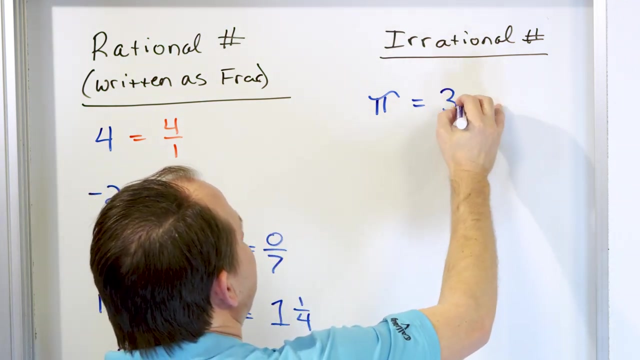 that pi can be calculated as 22 divided by seven And that's not true. So anybody ever told you that is wrong. It's, it's just not correct. It's a common misconception people have. You cannot find pi by 22 divided by seven. It's not true. Pi is a number that starts out with 3.14.. That's. 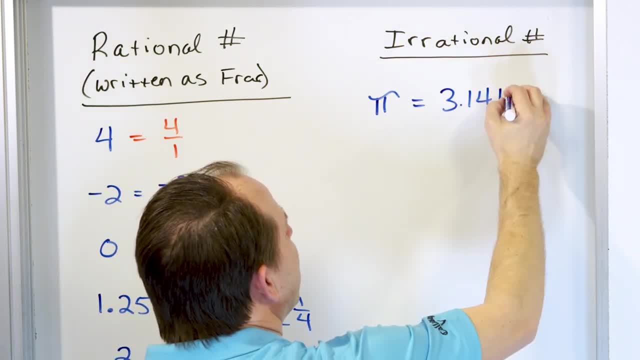 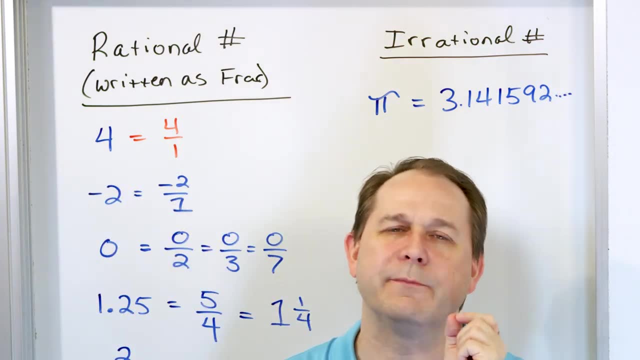 what we use in our calculations but actually goes on 3.141592.. And then it goes on and on forever. but there is no pattern to these decimals. In fact, people have used computers to calculate pi to millions of decimal places, And I mean literally millions of decimal places. 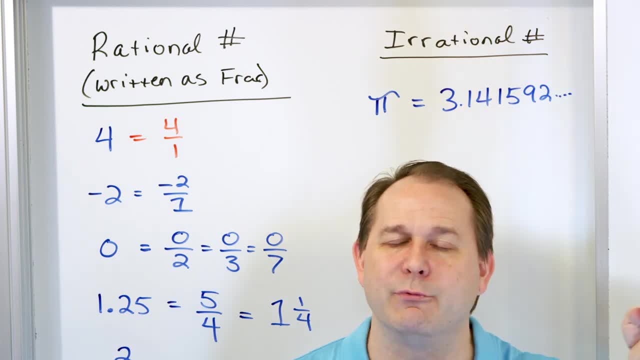 And, as far as we can tell, there is no pattern in the decimal digits of pi. They go on forever, but there is no pattern to them, And that means that this number, pi, cannot be written as a ratio of two whole numbers, a fraction that involves two whole numbers, like this: Okay, All right, What are 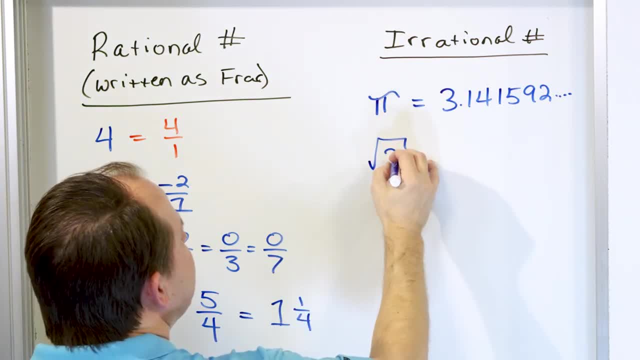 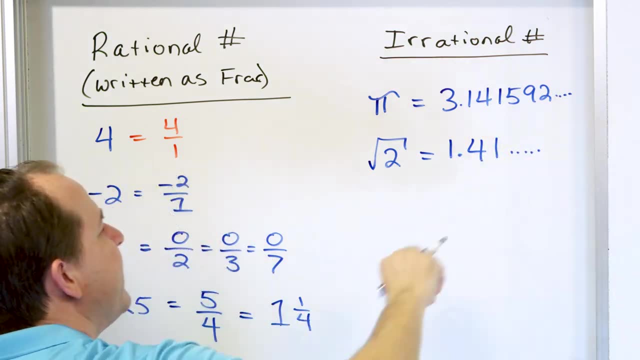 some other irrational numbers. It turns out that the square root of the number two is also irrational, And if you put that in the calculator you're going to get 1.41, and then a bunch of digits after it that don't have any pattern to that. that you can, that you can see Also just 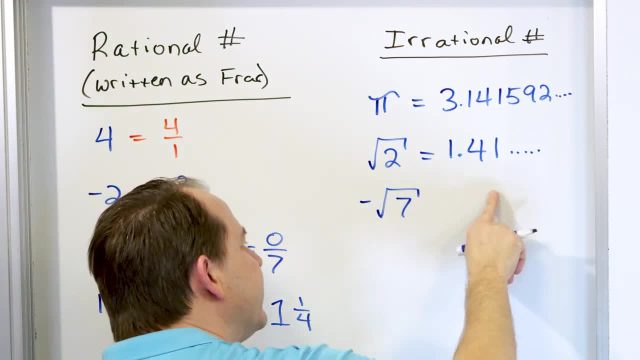 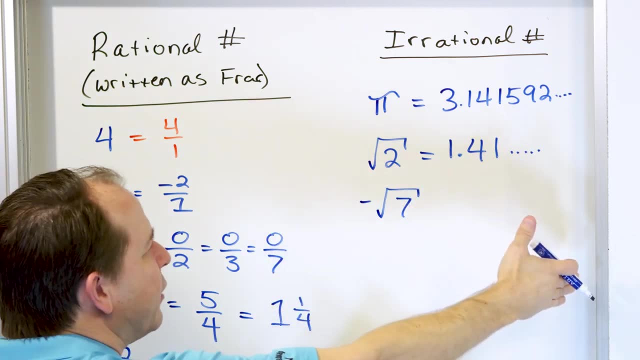 another example: negative square root of seven. If you put that in a calculator you're going to find that there's a decimal, a decimal you know, negative decimal pattern to it, but there is no pattern. It goes on and on forever in your calculator window, but there is no pattern to it. 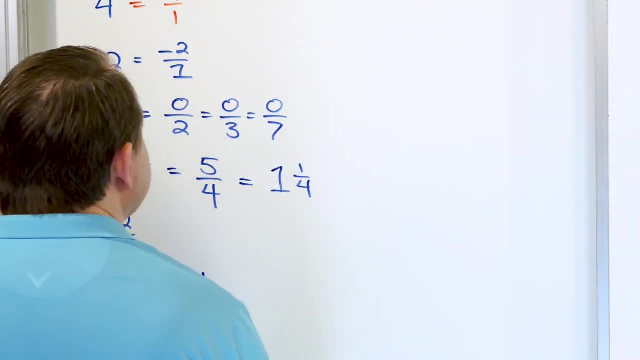 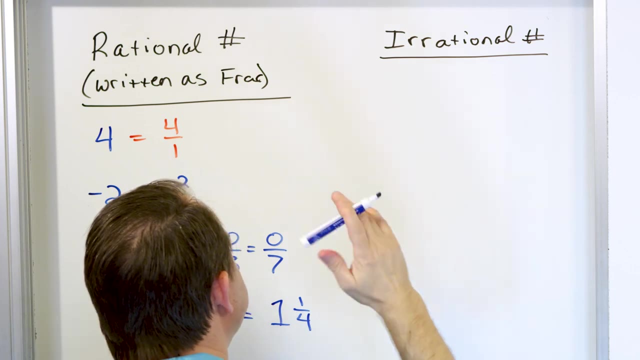 there's a pattern. So let's give some examples of the, some numbers that are irrational. Well, the most famous one that you're all aware of, the, the, the granddaddy of all of them, is the number pi. Some people may have told you incorrectly that pi 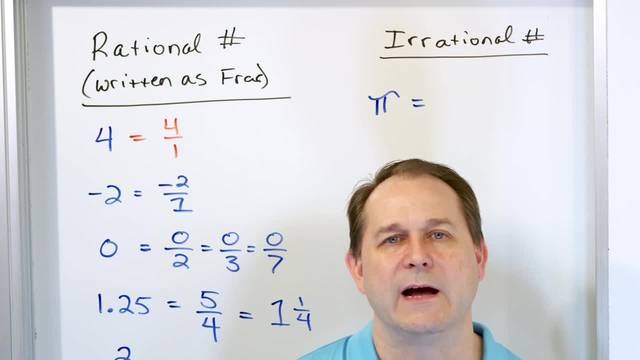 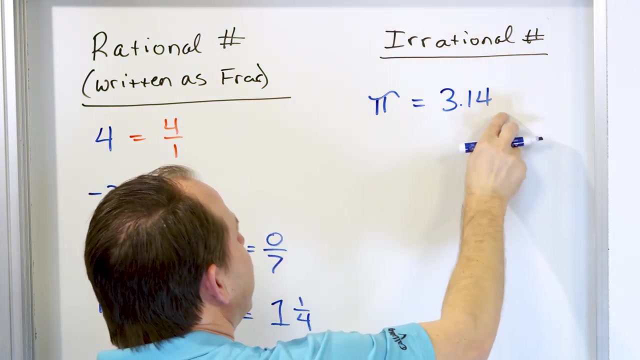 can be calculated as 22 divided by 7, and that's not true. So anybody ever told you that is wrong. It's, it's just not correct. It's a common misconception people have. You cannot find pi by 22 divided by 7.. It's not true. Pi is a number that starts out with 3.14.. That's what. 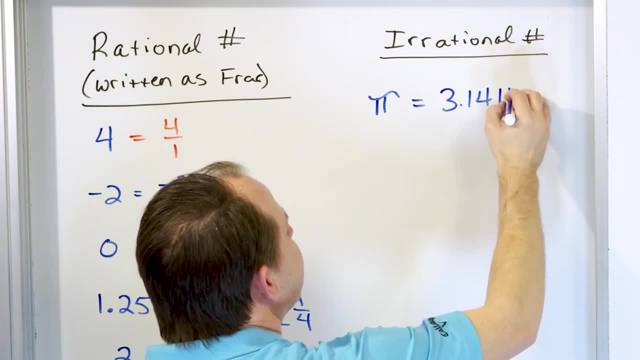 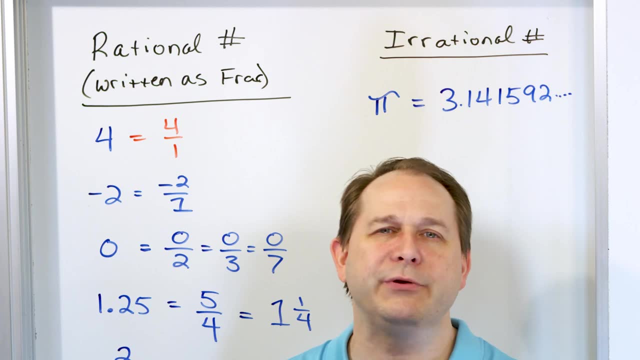 we use in our calculations, but it actually goes on 3.141592, and then it goes on and on for a forever, but there is no pattern to these decimals. In fact, people have used computers to calculate pi to millions of decimal places, and I mean literally millions of decimal places, and as far 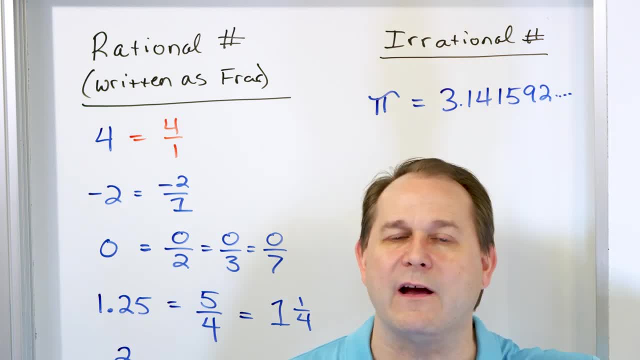 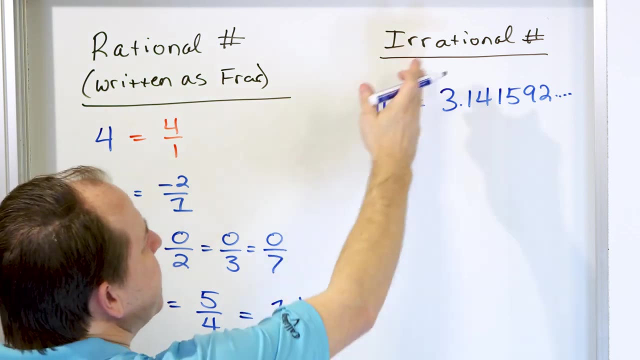 as we can tell, there is no pattern in the decimal digits of pi. They go on forever, but there is no pattern to them, and that means that this number, pi, cannot be written as a ratio of two whole numbers, a fraction that involves two whole numbers, like this: okay, All right, what are some other? 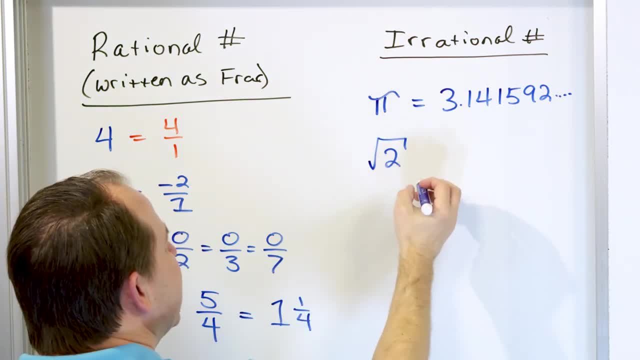 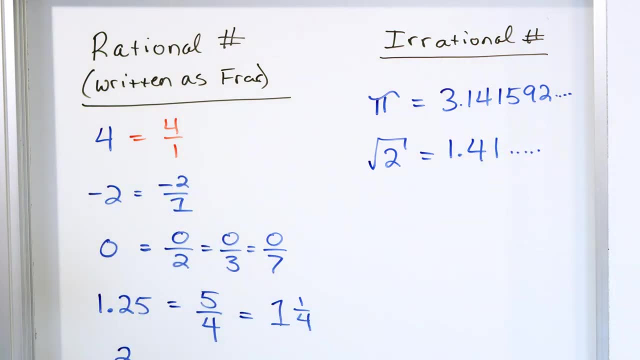 rational numbers. It turns out that the square root of the number 2 is also irrational and if you put that in a calculator you're going to get 1.41 and then a bunch of digits after it that don't have any pattern to it. that you can, that you can see Also. just another example: negative square. 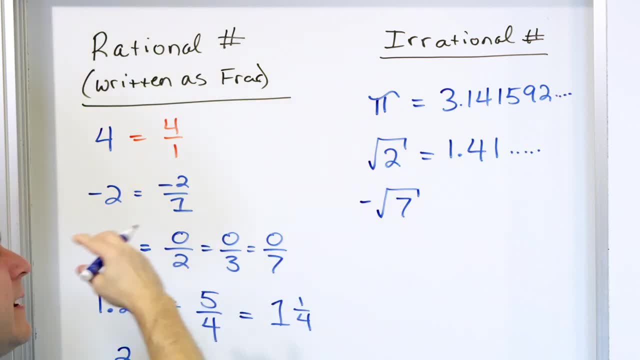 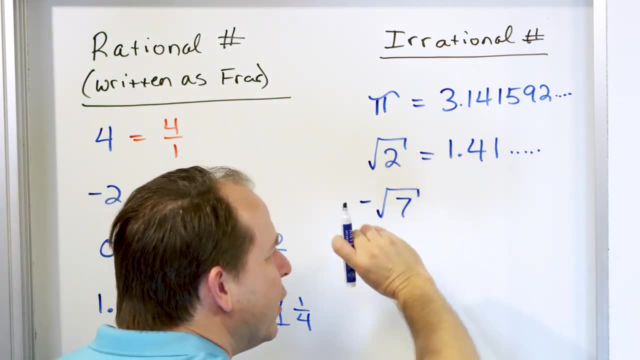 root of 7.. If you put that in a calculator you're going to find there's a decimal, a decimal you know, negative decimal pattern to it, but there is no pattern. It goes on and on forever in your calculator window but there is no pattern to it. So basically, 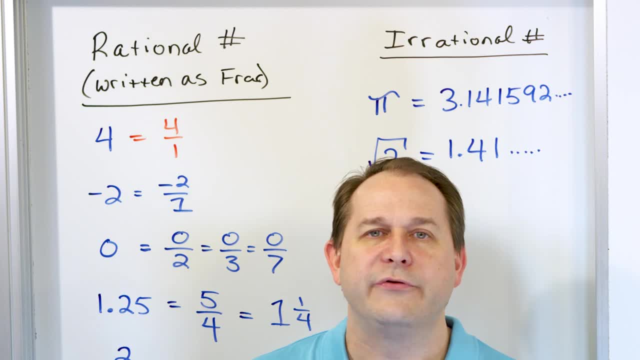 the radicals that you know, the square roots that give you whole numbers. those are rational because they give you whole number answers. but all the other radicals that don't give you whole number answers, they're going to be irrational If you take square root of 3 and put it in a calculator. 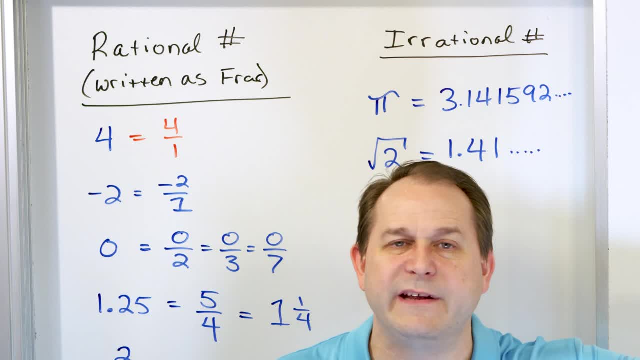 then it's going to give you a number- you know one point, and then some digits after it that do not repeat. There's no pattern to it. You know, we know, the square root of 4 is 2, but the square 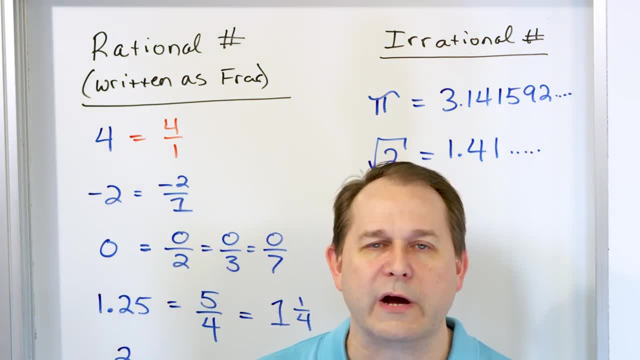 So basically, the radicals that you know, the square roots that give you whole numbers, those are rational because they give you whole number answers. But all the other radicals that don't give you whole number answers, they're going to be irrational. If you take square root of three, 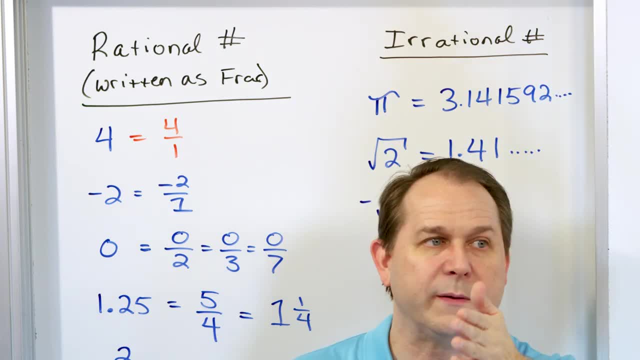 and put it in a calculator, then it's going to give you a number- you know one point, and then some some digits after it that do not repeat. There's no pattern to it. You know, we know, the square root of four is two, but the square root of five is irrational. It goes on and on forever. 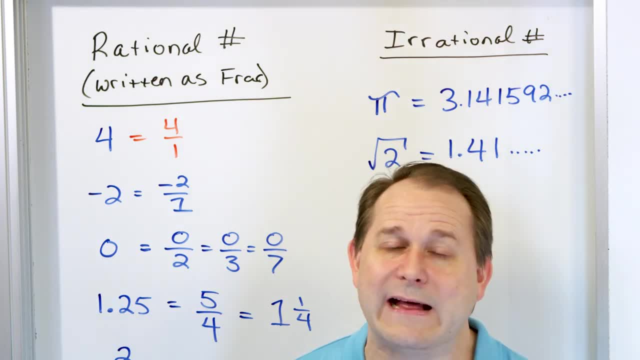 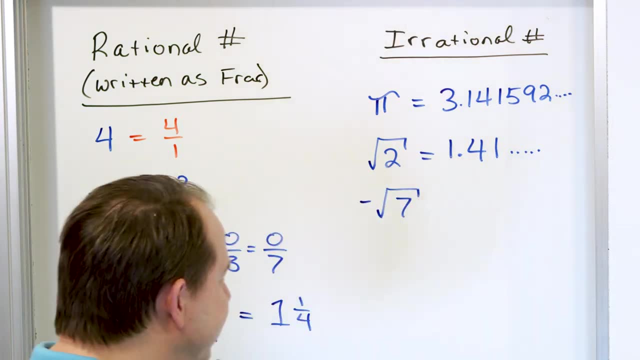 The square root of six is irrational. We know the square root of nine is three, That's perfect square. But the square root of 10 is irrational. It goes on and on forever in the calculator window like this. So let's summarize: We have two main 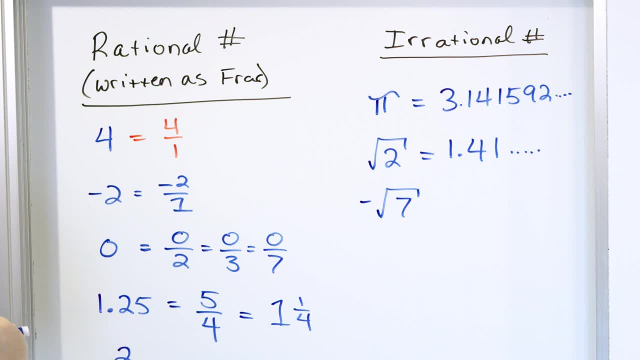 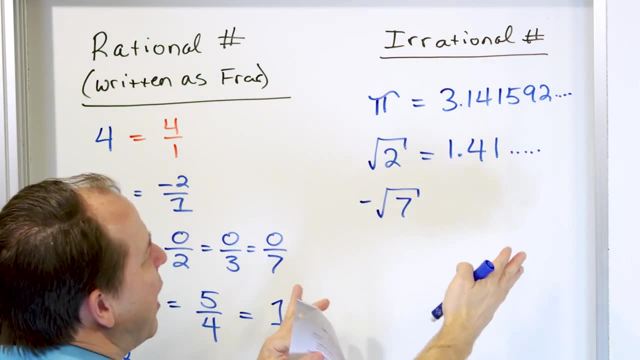 classes of numbers. in math We have the rational numbers and the irrational numbers. The rational numbers can be written as a fraction and the irrational numbers cannot. The irrational numbers are easier to talk about because there's really not that much to say. It's just a decimal that. 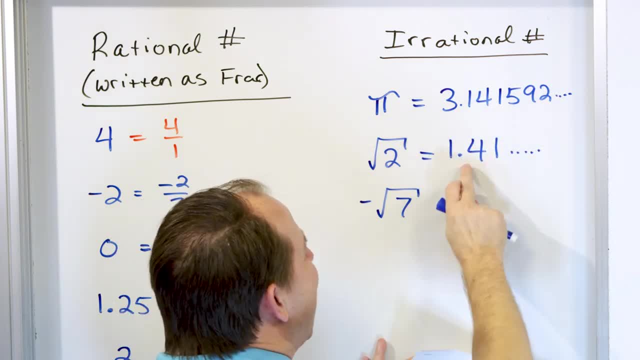 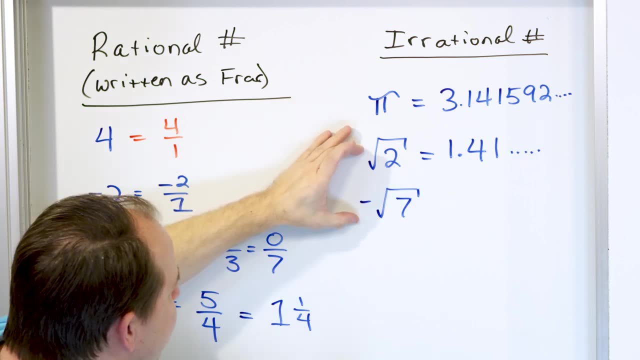 goes on and on forever, with no pattern in the, in the numbers after the decimal point, And the number pi is the most famous of these irrational numbers. Any radical like a square root that you, that you calculate, that isn't a perfect answer. with a, with a whole number, is. 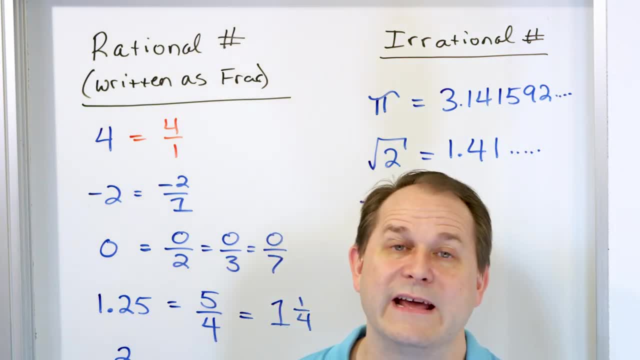 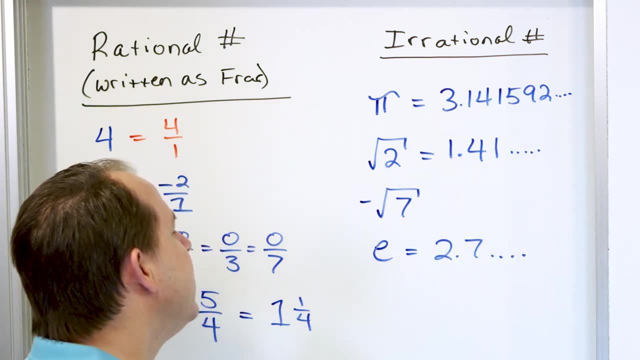 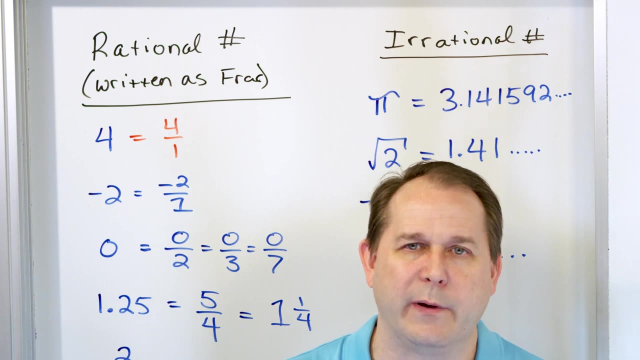 going to be an irrational number as well. There are other numbers in math that are irrational. There's a famous number called E, which is 2.7, and a bunch of digits after it, And that number shows up a lot in exponential growth, growth of money. It shows up everywhere actually. It's actually just 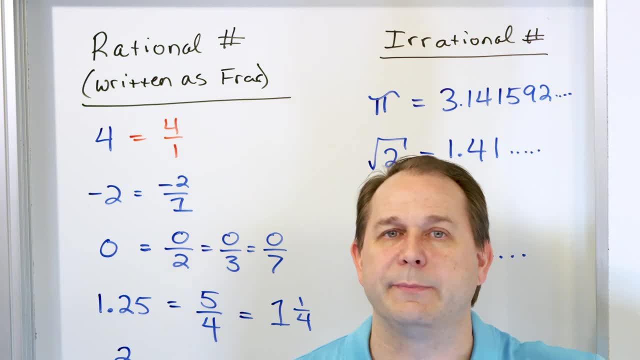 important as pi. You just don't learn about the number e until a little bit later in math, But it's on equal footing with pi. e shows up everywhere And it's a number that's 2.7, and then there's digits after it. that goes on and on forever, but there's no pattern to those. 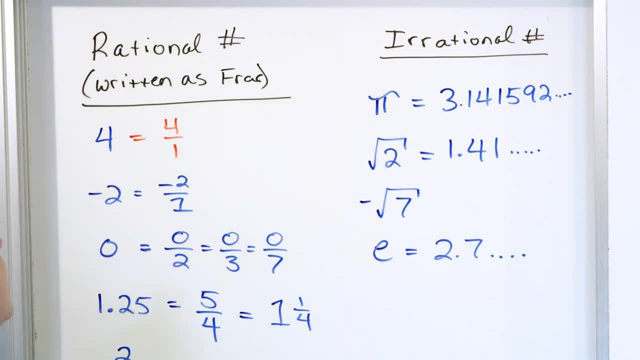 digits. You cannot write any of these numbers as a fraction, But all of these numbers can be written as fractions. The whole numbers can be written as fractions. The negative whole numbers can be written as fractions. Zero can be written as a fraction. Any decimal that just stops and 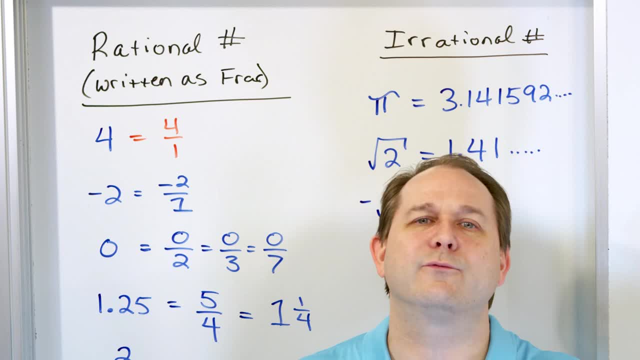 root of 5 is irrational. It goes on and on forever. The square root of 6 is irrational. We know the 3, that's perfect square. but the square root of 10 is irrational. It goes on and on forever in the 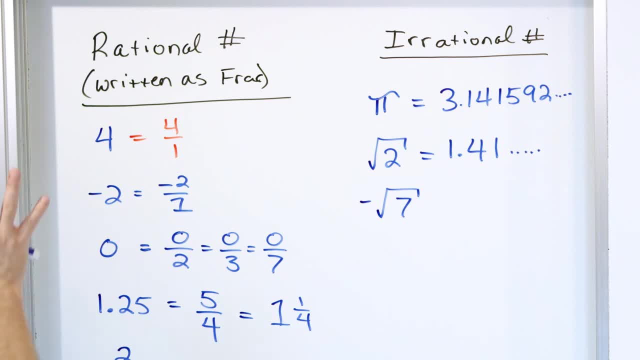 calculator window like this. So let's summarize: We have two main classes of numbers in math. We have the rational numbers and the irrational numbers. The rational numbers can be written as a fraction and the irrational numbers cannot. The irrational numbers are easier to talk about. 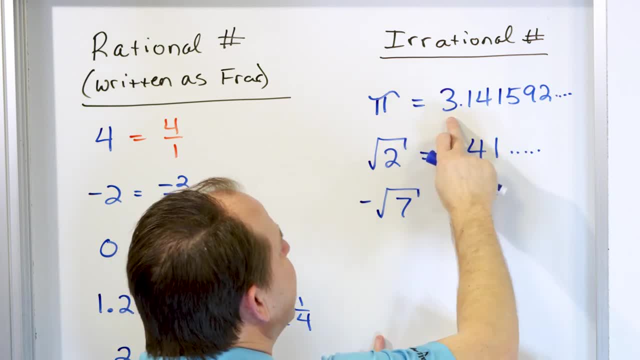 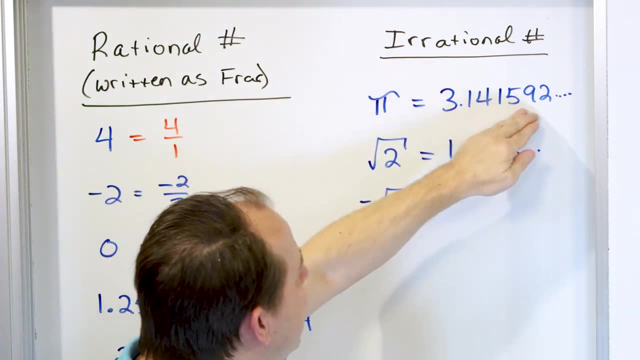 because there's really not that much to say. It's just a decimal that goes on and on forever, with no pattern in the numbers after the decimal point. And the number pi is the most famous of these irrational numbers. Any radical like a square root. 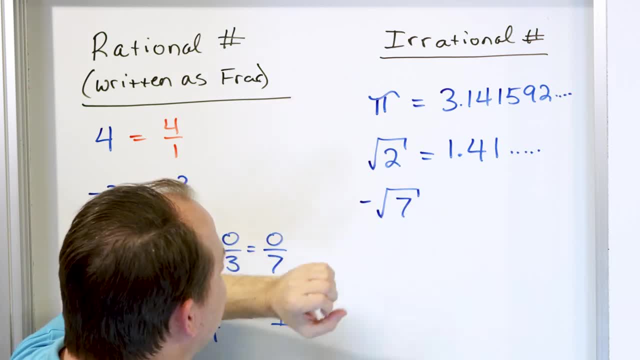 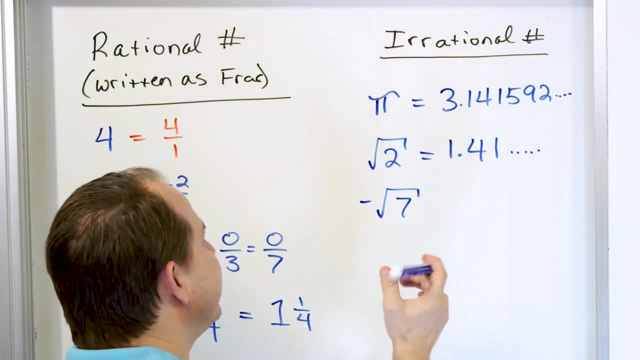 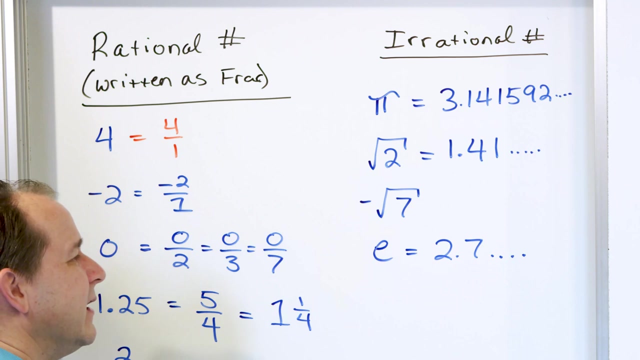 that you calculate. that isn't a perfect answer, with a whole number is going to be an irrational number as well. There are other numbers in math that are irrational. There's a famous number called e, which is 2.7, and a bunch of digits after it, And that number shows up a lot. 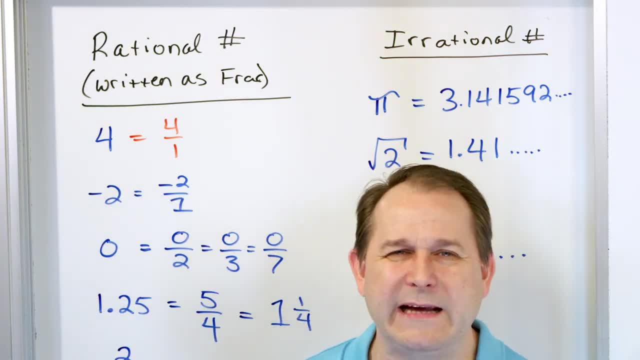 in exponential growth, growth of money. It shows up everywhere actually. It's actually just as kind of what theılKE, which means two, because it's the number the plus. You just don't learn about the number e until a little bit later in math. But it's just as it's, on equal footing with 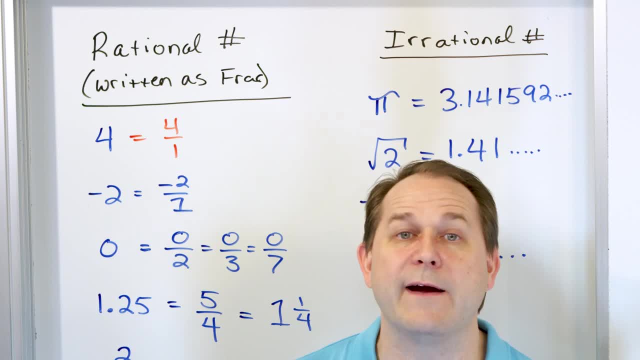 pi E shows up everywhere And it's a number that's 2.7.. And then there's digits after it. that goes on and on forever. but there no pattern to those digits. You cannot write any of these numbers as a fraction. But all of these numbers can be written as fractions. The whole numbers can. 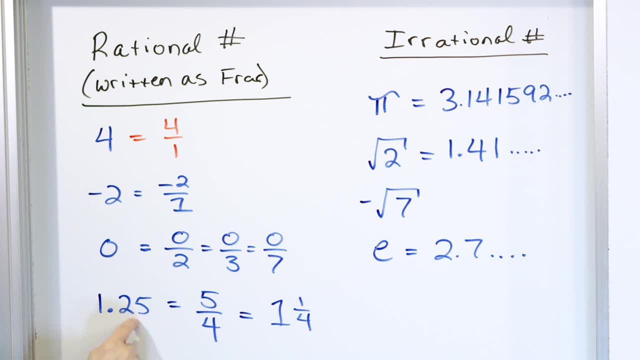 be written as fractions. The negative whole numbers can be written as fractions. Zero can be written as a fraction Number At like z by A R Z. Any decimal that just stops in its tracks can always be written as fractions. That can always be perfect without no middle number. for that It's a contradiction. 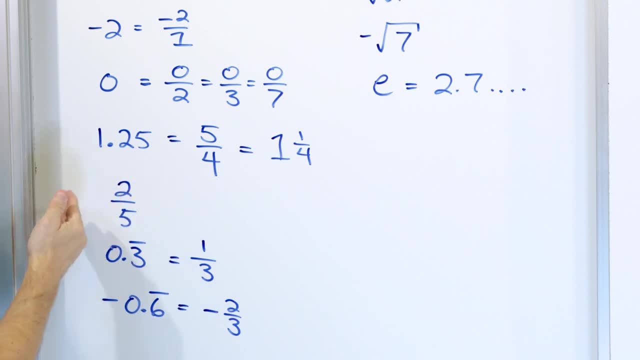 tracts can always be written as a fraction. The fractions that you know and love from fourth grade are all written as fractions. Any decimals that go on and on forever but have a pattern, like any of these repeating decimals, you can write them as fractions as well, And even examples. I 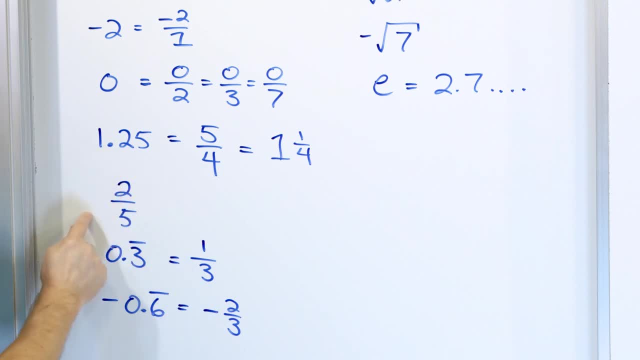 it's tracked can always be written as a fraction. The fractions that you know and love from fourth grade are all written as fractions. Any decimals that go on and on forever but have a pattern, like any of these repeating decimals, you can write them as fractions as well, And even examples. I 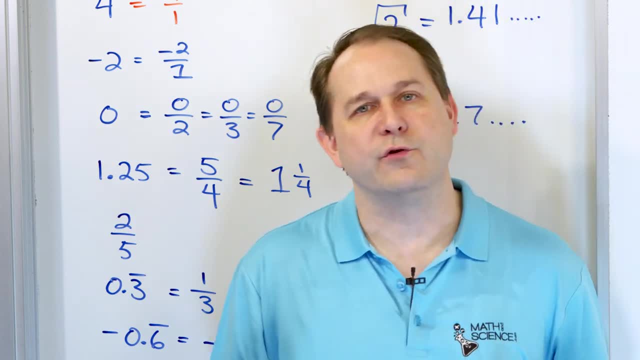 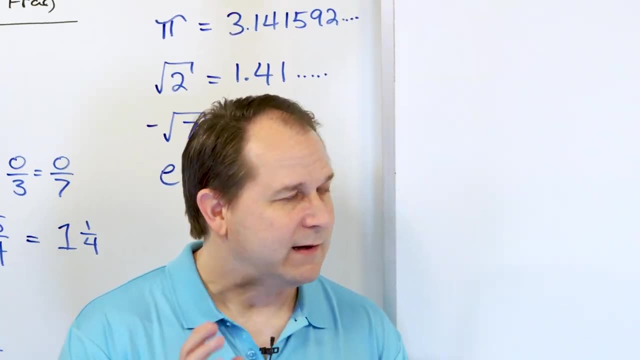 gave you like 5.321,, 321,, 321,. if there's a pattern, it can be written as a fraction. It is rational, Everything else irrational. So let's start off by asking ourselves the following Are the following: 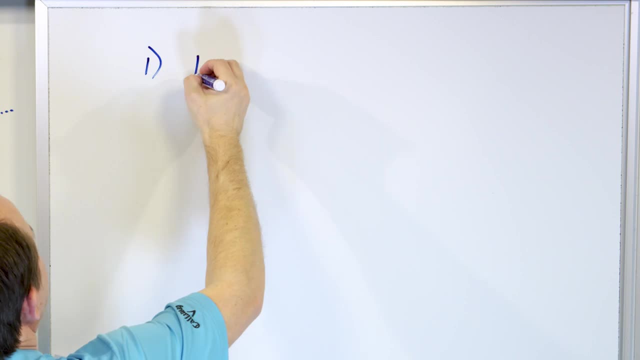 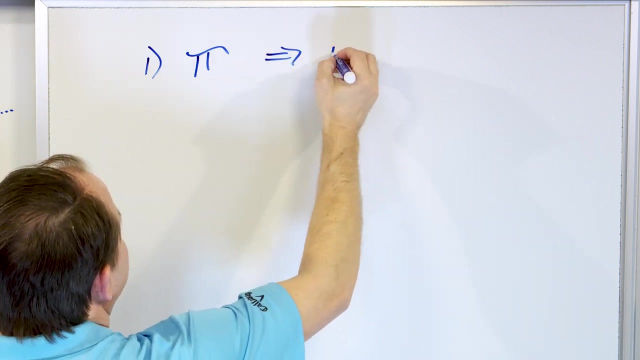 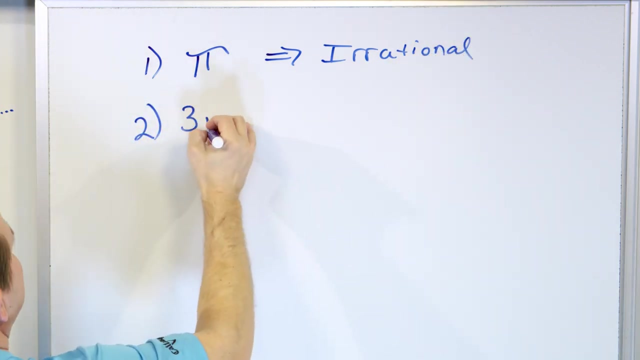 numbers Irrational or not? What about the number pi? Is it rational or irrational? We just told you it's an irrational number, So I'm going to put over here irrational, And I don't even have this in my notes. but let's look at three times pi. 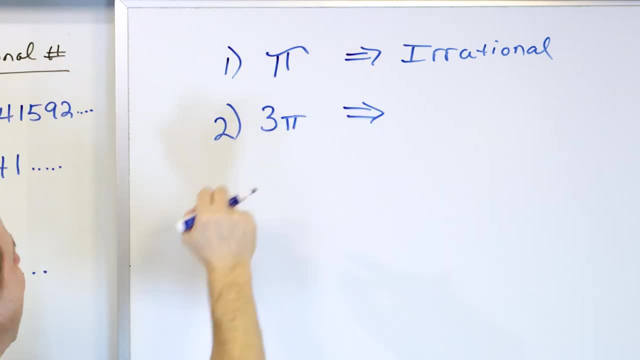 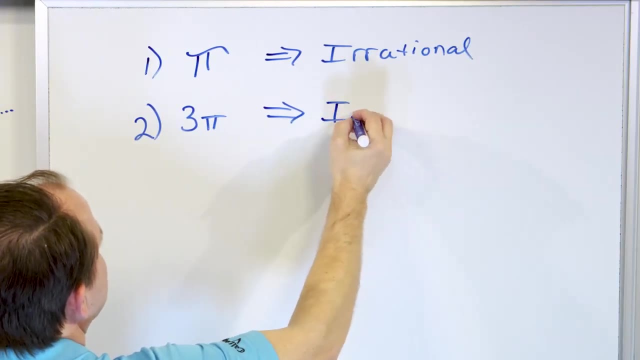 Is it irrational or rational? Well, if the number pi is irrational, if we take this number and multiply it by three, all of the decimals will be different, but there'll still be no pattern. It's also irrational, Right, Also irrational. Anything involving pi is always going to be irrational. What about the? 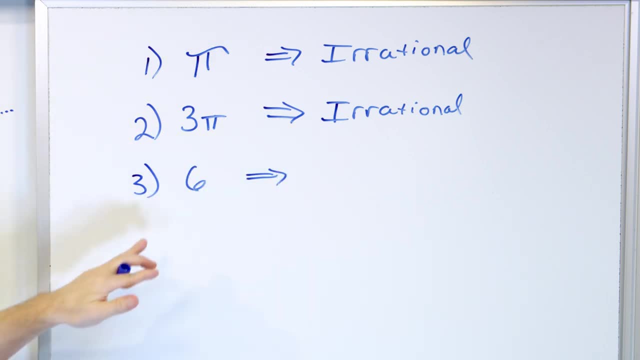 number six. Is it rational or irrational? Well, any of the whole numbers. I can write this as six over one. This is a rational number because I can write it as a fraction. What about the following Negative seven tenths? Well, it's already a fraction, It's negative. 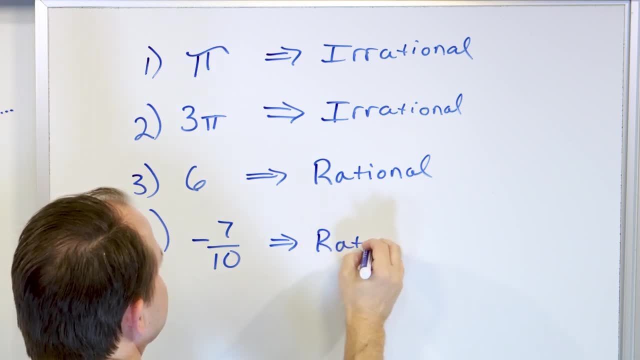 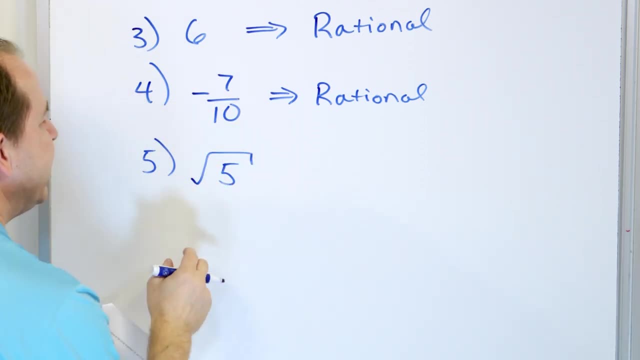 but that's okay, It's still a fraction. This is rational, All right. What about the square root of the number five? I said the square roots of the perfect squares, like square root of 16, to give you four. That, of course, is rational because 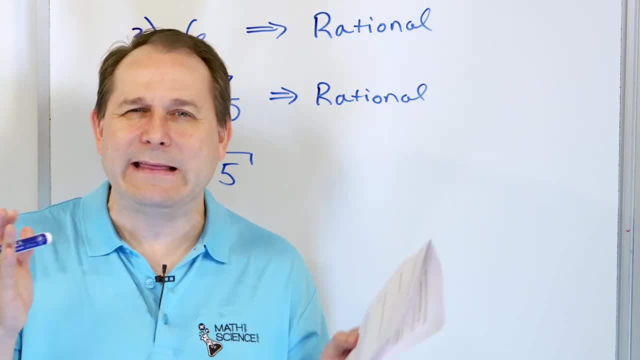 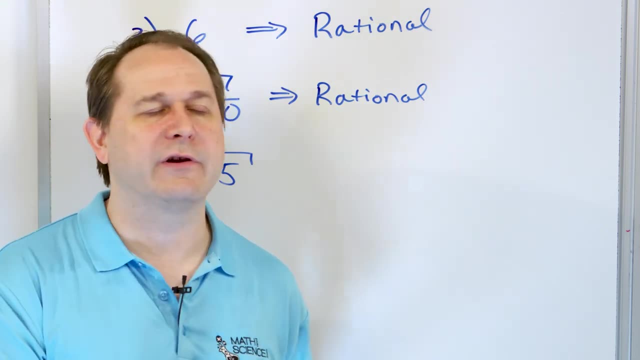 four, the answer is a whole number. But anything that's not a perfect square, like that, square root of five, square root of six, square root of seven, square root of eight, they're all going to give you decimals in the calculator that don't repeat. This obviously is not a perfect square, so it's. 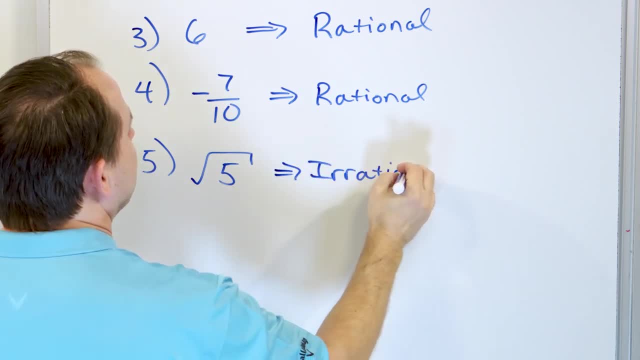 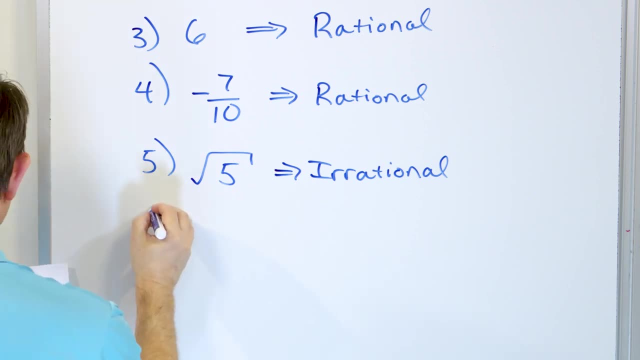 going to be irrational. Go ahead, grab a calculator and take the square root of five and see what you get. You'll see that it goes on and on forever. What about the number 2.68? This is a decimal. I don't know what the 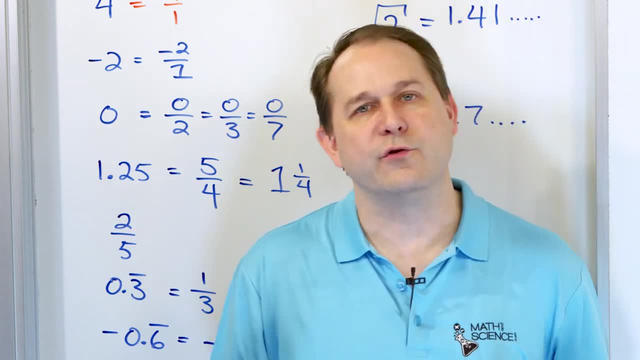 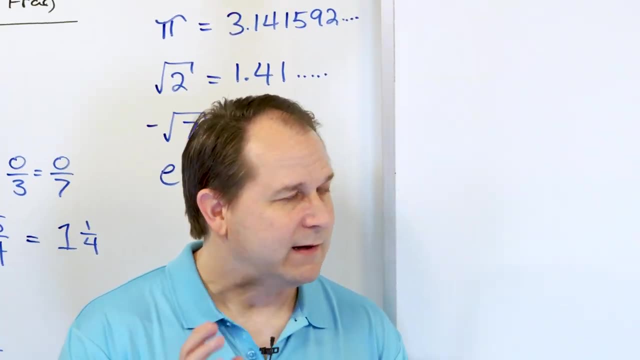 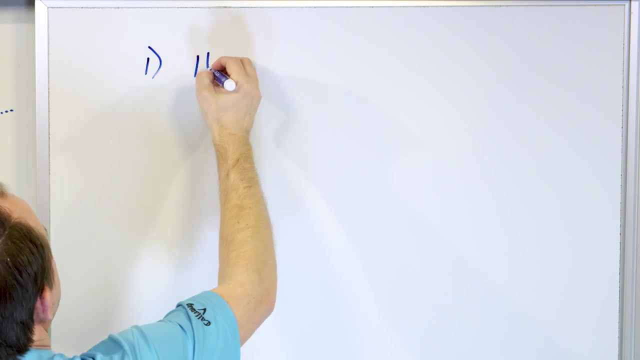 gave you like 5.321,, 321, 321,. if there's a pattern, it can be written as a fraction. It is rational, Everything else irrational. So let's start off by asking ourselves the following: Are the following numbers irrational or not? What about the number pi? Is it rational or irrational? 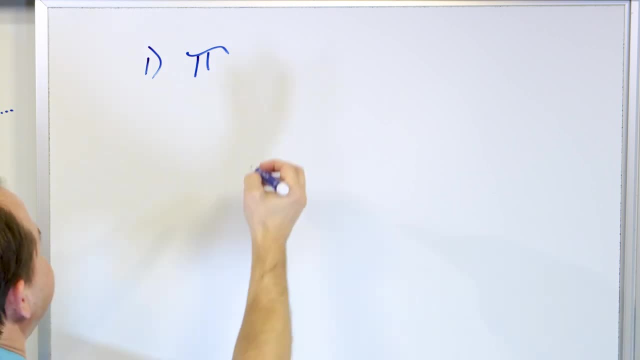 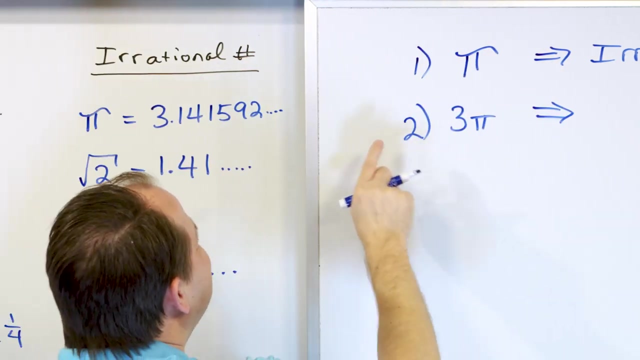 We just told you it's an irrational number, So I'm going to put over here irrational And I don't even have this in my notes. but let's look at three times pi. Is it irrational or rational? Well, if the number pi is irrational, if we take this number and 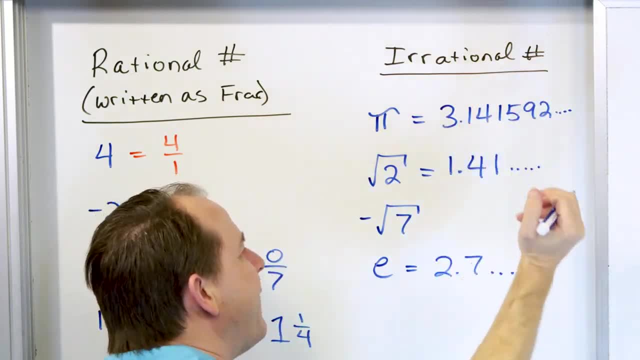 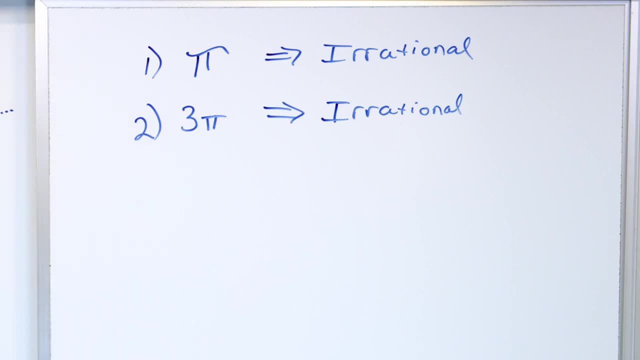 multiply it by three. all of the decimals will be different, but there'll still be no pattern. It's also irrational, Right? Oh, also irrational. Anything involving pi is always going to be irrational. What about the number six? Is it rational or irrational? Well, any of the whole numbers. I can write this: 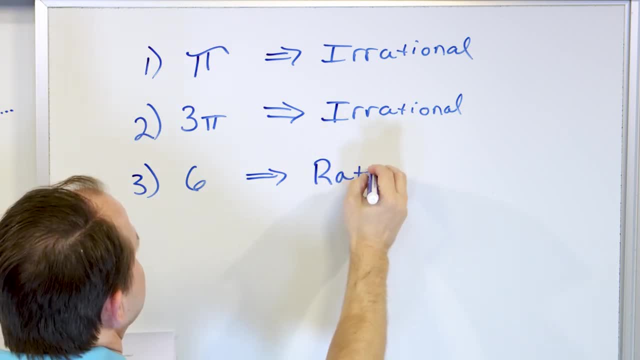 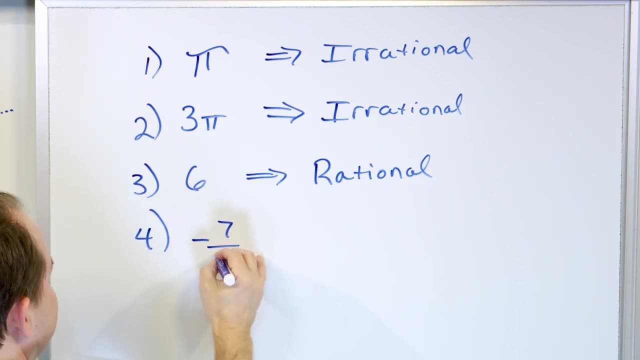 as six over one. This is a rational number because I can write it as a fraction. What about the following Negative seven tenths? Well, it's already a fraction. It's negative, but that's okay, It's still a fraction. This is rational. 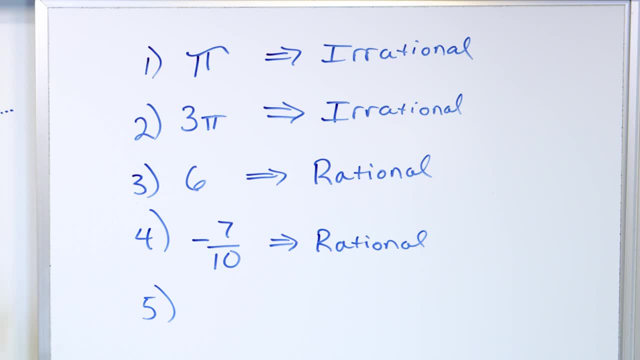 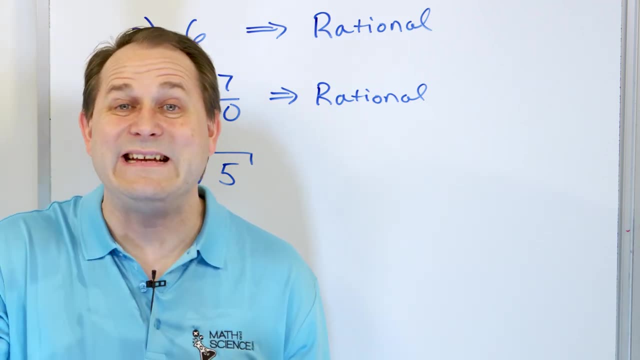 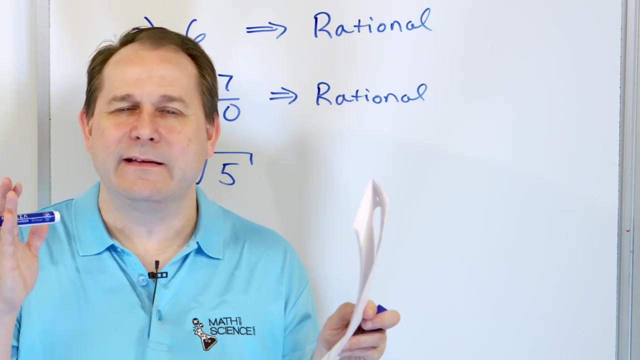 All right, What about the square root of the number five? I said the square roots of the perfect squares, like square root of 16, to give you four. That of course is rational, because four the answer is a whole number. But anything that's not a perfect square like that square root. 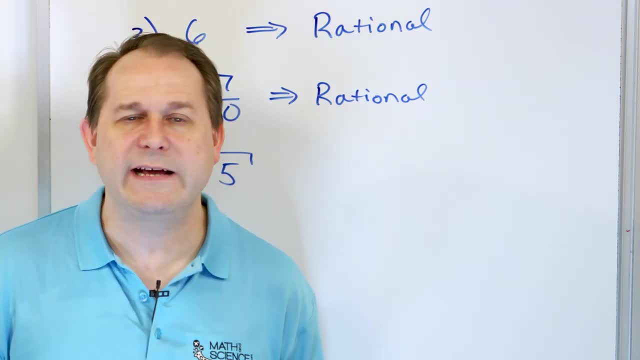 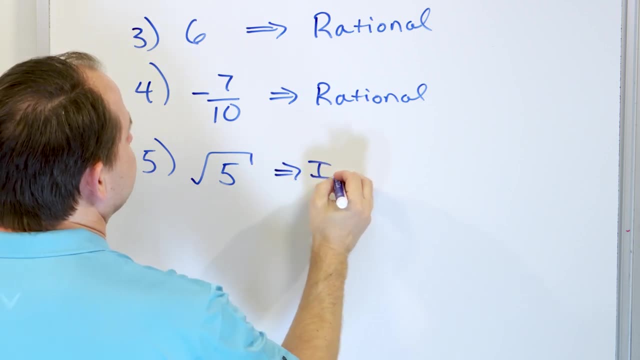 of five, square root of six, square root of seven, square root of eight. they're all going to give you decimals in the calculator that don't repeat. This obviously is not a perfect square, so it's going to be irrational. Go ahead, grab a calculator and take the square root of five and see what you get. You'll see that. 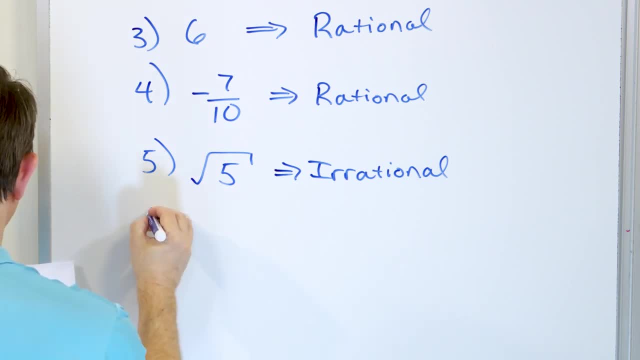 it goes on and on forever. What about the number 2.68?? This is a decimal. I don't know what the fraction is off the top of my head, but I know that it's a decimal. that stops. All right, And so. 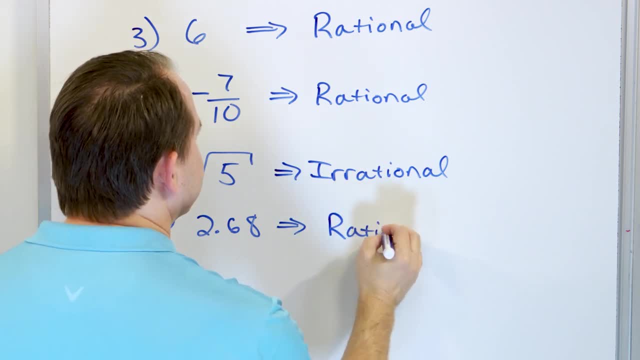 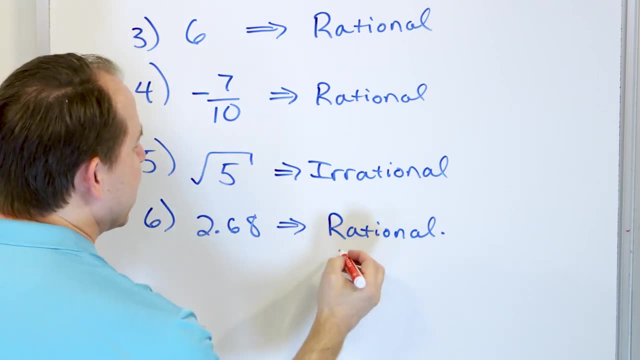 I know that this is rational. In fact, we can write it as a fraction right now. Think about it: When you divide, you get a decimal. When you divide, you get a decimal. When you divide, you get a decimal. When you divide by 100, you move the decimal right. We can write this as 268 divided by. 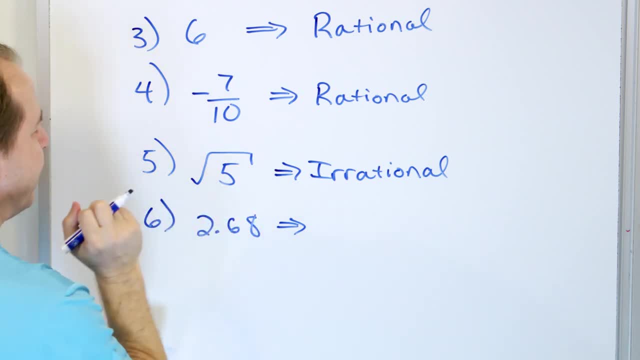 fraction is off the top of my head, but I know that it's a decimal. that stops All right, And so I know that this is rational. In fact, we can write it as a fraction right now. Think about it: When you divide by 100, you move the decimal. 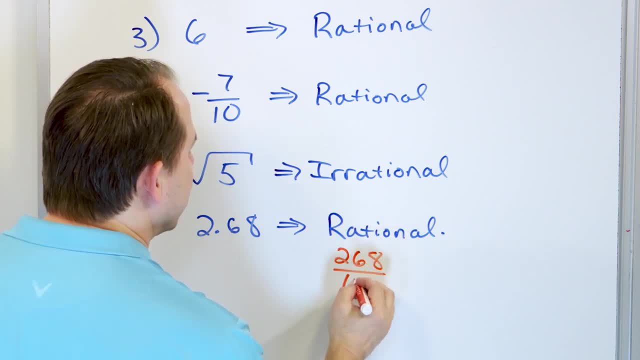 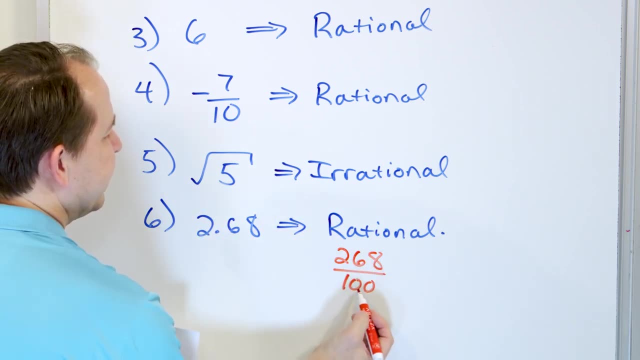 We can write this as 268 divided by 100.. All that's going to do is take the decimal here and move it two spots to the left, So 2.68,. we can write it as 268 over 100, because that's going to. 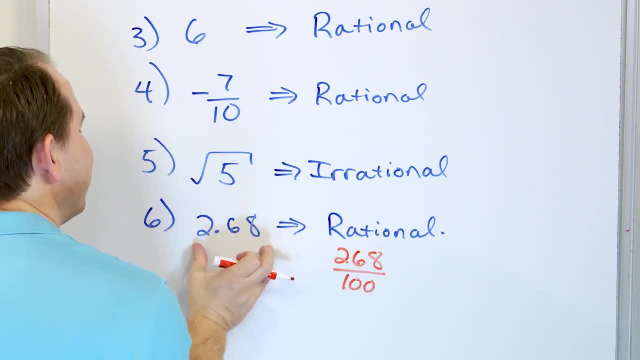 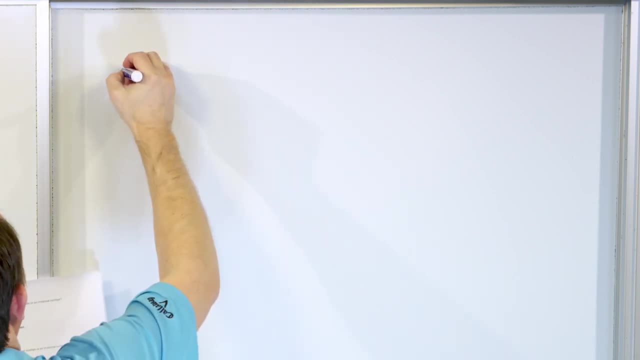 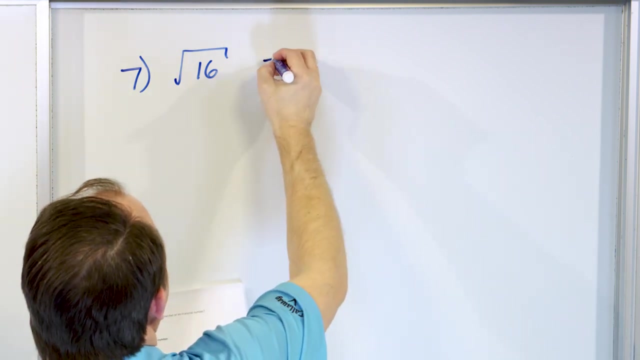 give us this. So this, of course, is a fraction representation of this guy right here. What about the square root? Let's look at the number seven, The square root of 16, is this rational or irrational? Well, we know that this has got to. 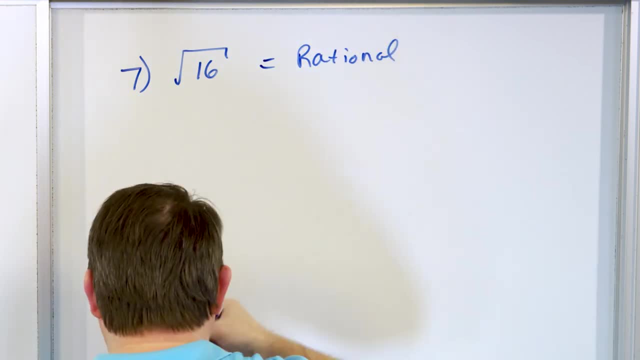 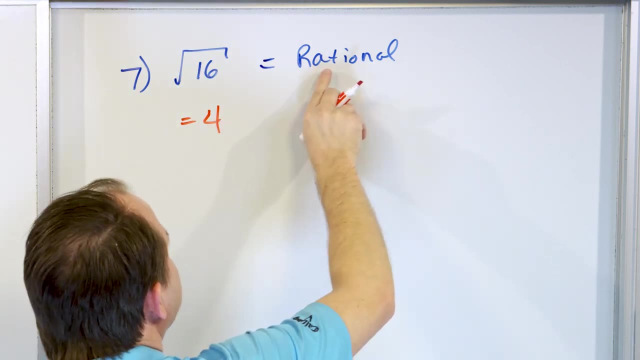 be rational. How do we know that? Because if we try to calculate what the square root of 16 is, we already know the answer is four, because four times four is 16 and four is a whole number. And so since these two things are equal, we know the answer has to be rational. 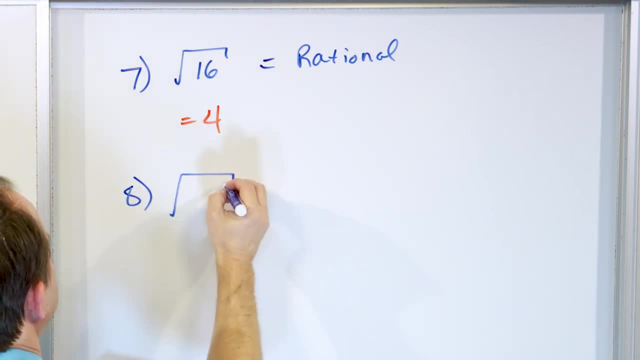 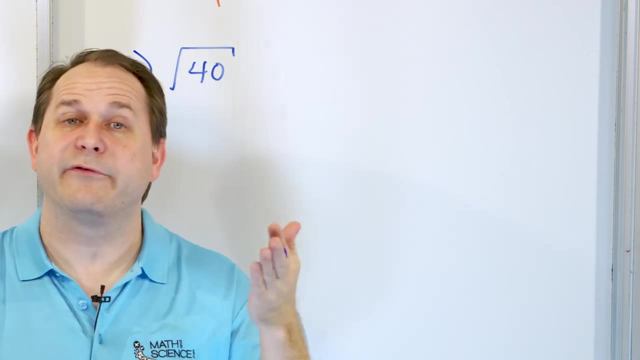 And then, finally, let's take a look at the square root of 40.. Now, you may not know what the square root of 40 is, but we can start thinking right. Okay, So let's go up Three times three is nine. 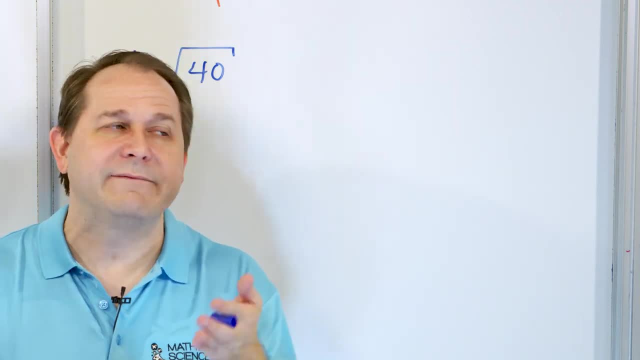 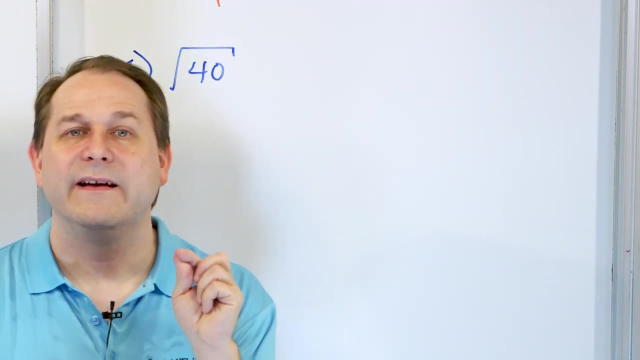 That's not right. Four is 16.. That's not right. Five times five is 25.. That's getting closer, but it's not big enough. Six times six is 36.. That's almost as big as that. Seven times seven: 49.. That's too big. 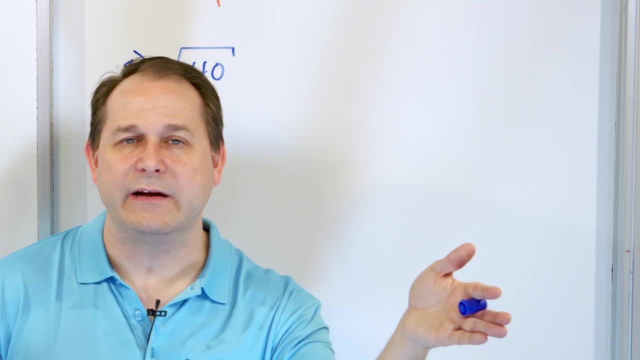 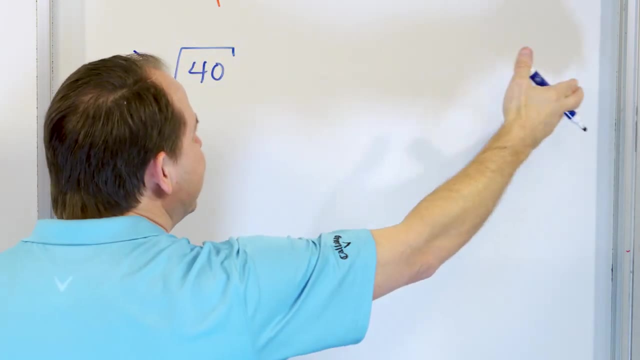 So we know that the answer to this thing cannot be six and it cannot be seven. It's got to be somewhere between six and seven, And when you put that in a calculator you're going to find out that you'll get six point something, and the digits will go on and on forever. 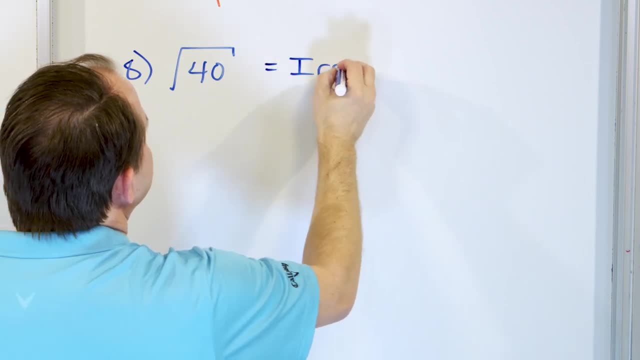 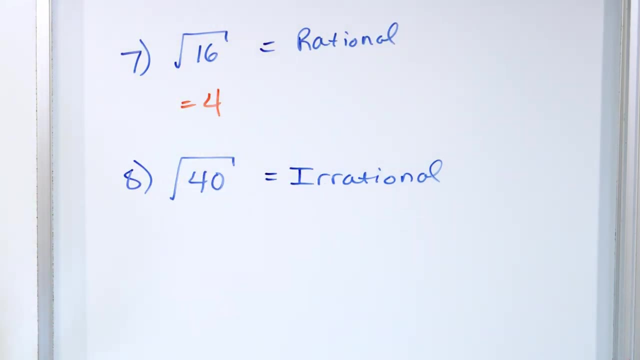 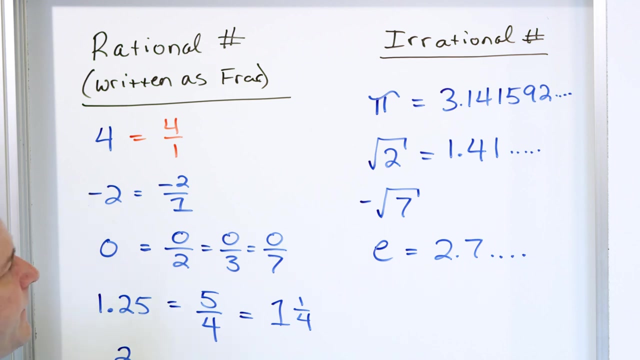 and they will not repeat, And so this is going to be irrational. So when you get a radical, if you get a whole number, it's rational. Otherwise it's basically always irrational like this. So the idea here is for us to understand a little bit more about. 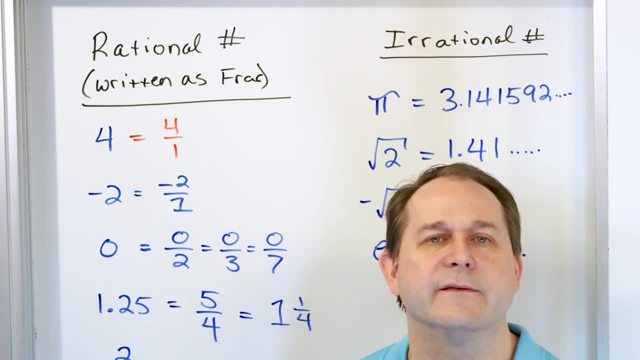 radicals, because we're going to be using radicals a lot in the next few lessons And so we have to do a kind of a global step back lesson here to talk about what a rational and an irrational number is. And basically it goes as follows: Almost every number is irrational, And so we're 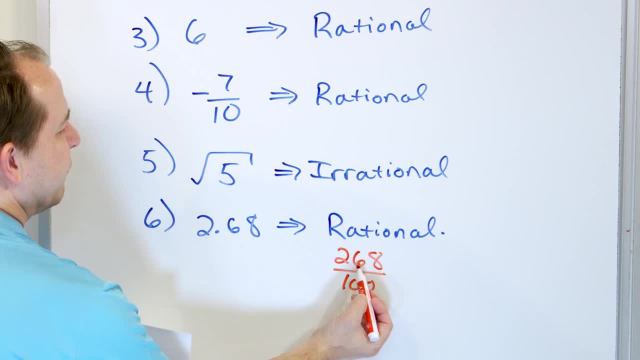 100.. All that's going to do is take the decimal here and move it two spots to the left, So 2.68, we can write it as 268 over 100, because that's going to give us this. So this, of course, is a. 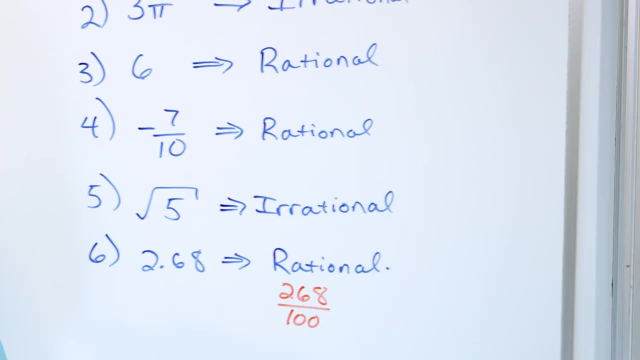 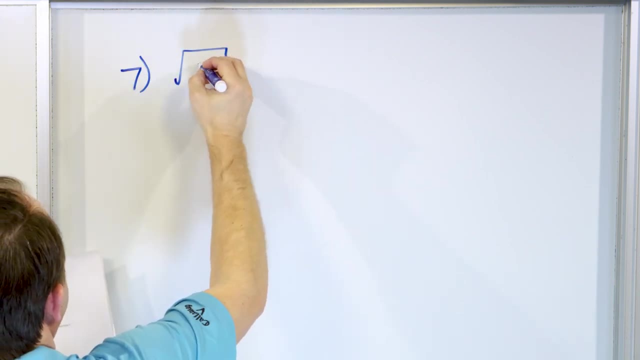 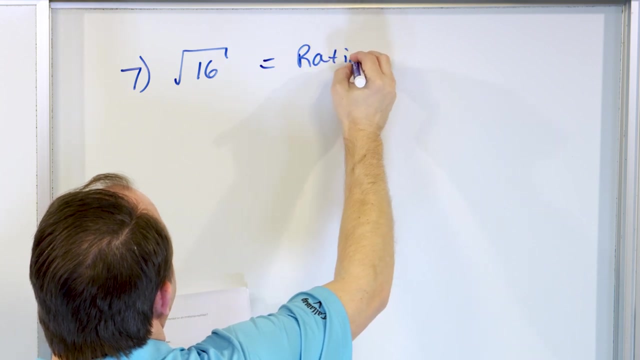 fraction representation of this guy right here. What about the square root? Let's look at the number seven, The square root of 16, is this rational or irrational? Well, we know that the number is equal, that this has got to be rational. How do we know that? Because if we try to 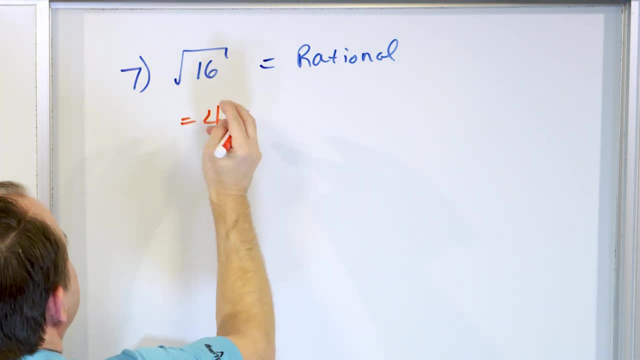 calculate what the square root of 16 is. we already know the answer is four, because four times four is 16 and four is a whole number. And so since these two things are equal, we know the answer has to be rational. And then, finally, let's take a look at the square root of 40.. Now you may not know what. 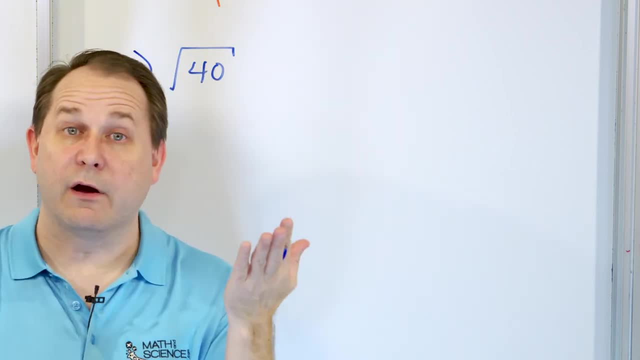 the square root of 40 is. but we can start thinking right, Okay, So let's go up. Three times three is nine, That's not right. So let's go up. three times three is nine. That's not right So. 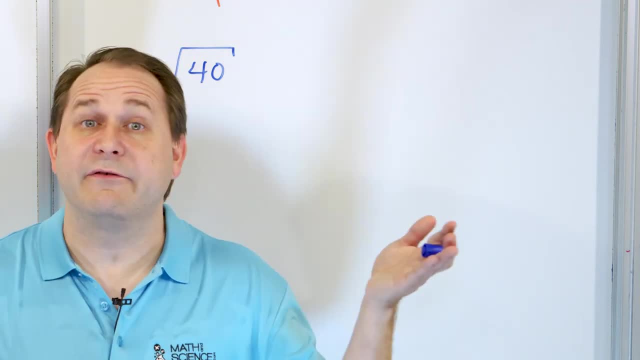 let's go up. three times three is nine. That's not right. Four times four is 16.. That's not right. Five times five is 25.. That's getting closer, but it's not big enough. Six times six is 36.. That's. 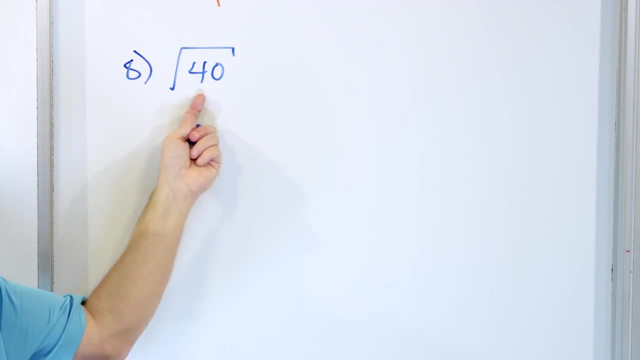 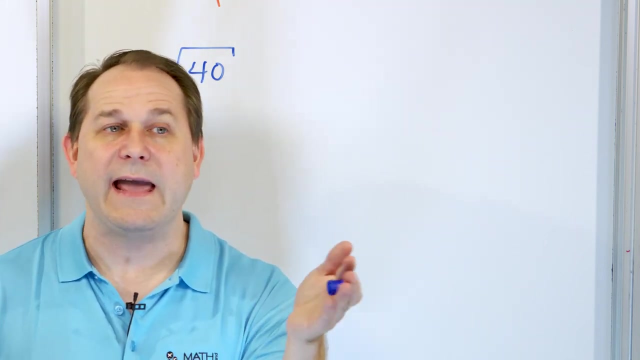 almost as big as that. Seven times seven, 49. That's too big. So we know that the answer to this thing cannot be six and it cannot be seven. It's got to be somewhere between six and seven And when you put that in a calculator you're going to find out that you'll get six point. 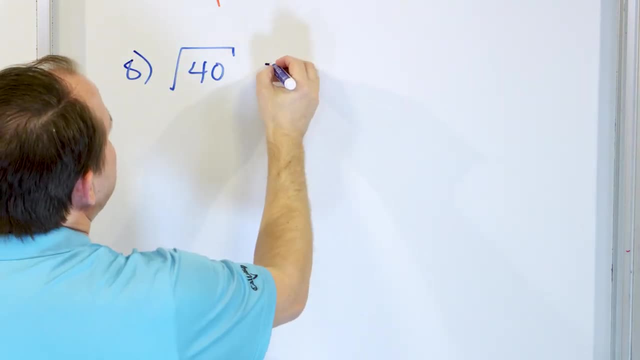 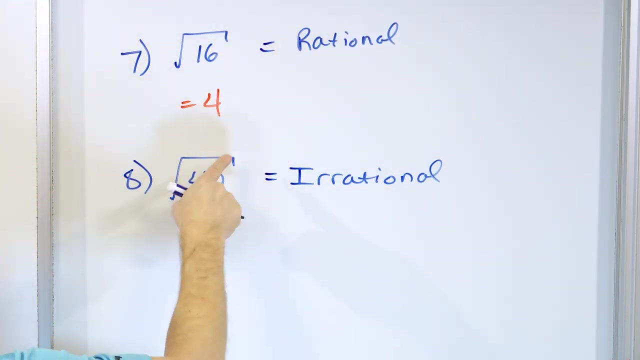 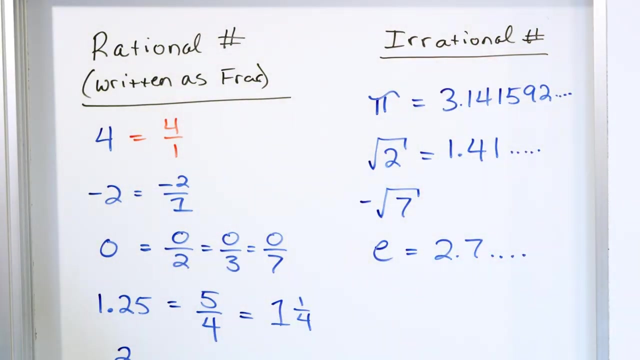 something and the digits will go on and on forever and they will not repeat, And so this is going to be irrational. So when you get a radical, if you get a whole number, it's rational. Otherwise it's basically always irrational like this. So the idea here is for us to understand a little bit more about. 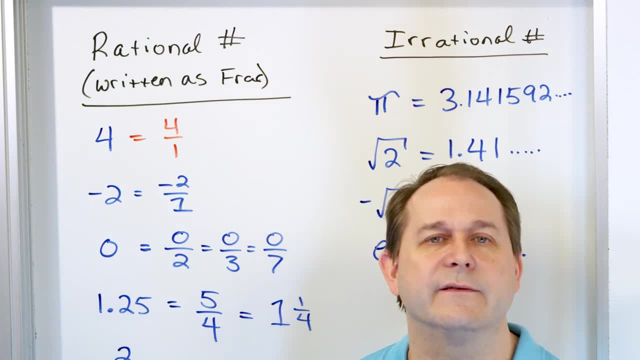 radicals, because we're going to be using radicals a lot in the next few lessons And so we have to do a kind of a global step back lesson here to talk about what a rational and an irrational number is. And basically it goes as follows: Almost everything you know and work with in real life- 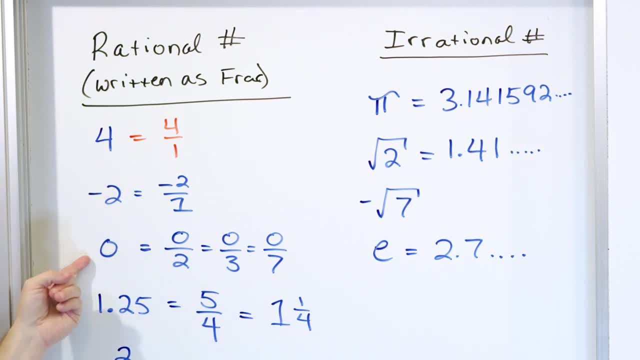 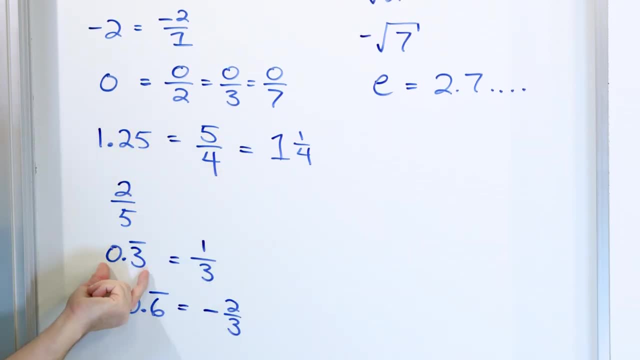 is rational. The whole number is irrational. The negative whole number is irrational. Zero is rational. Any decimal that stops is rational. Any fraction is rational. Any decimal that goes on forever with a pattern is rational. And everything else are just the weird oddball numbers They're.